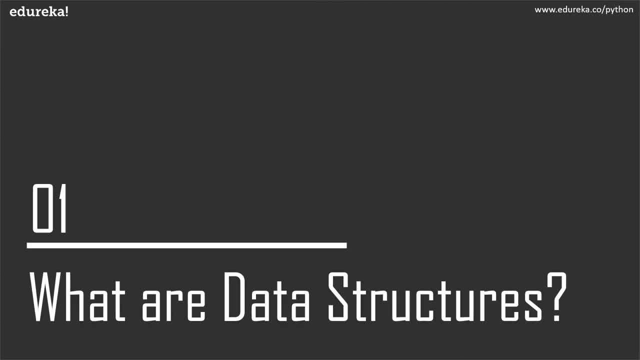 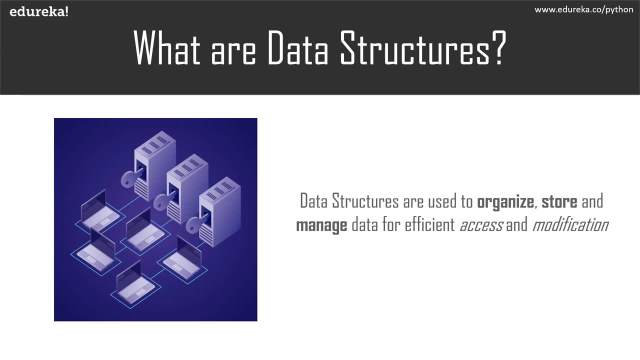 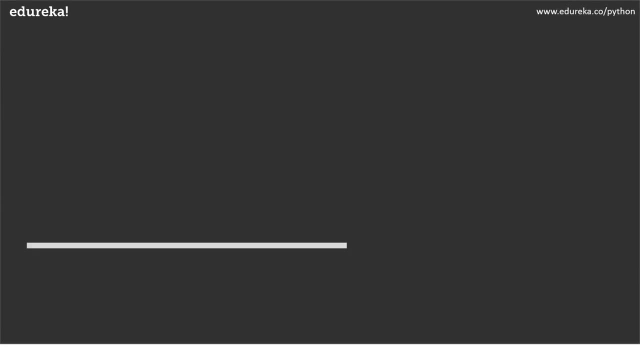 today's session. So the first topic for today: what is a data structure? So, as the definition suggests, it is a structure used to store, organize and manage data. It helps in better access to the data, which in turn, reduces the time required to solve a problem. So why is a data? 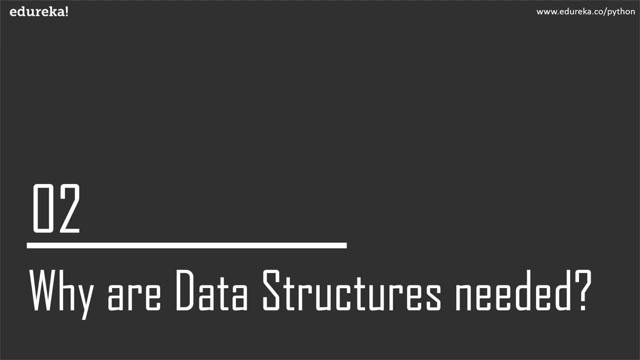 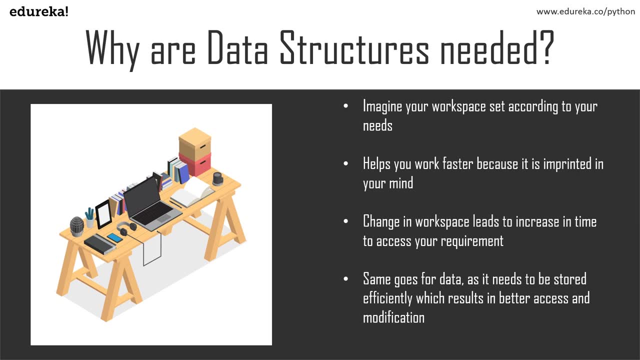 structure needed. Let us understand that with a simple example. Suppose you are at a workplace where you have Devices, cables, access points to ports set up according to your requirements. Your brain has imprinted this setup into itself, And so if you want to access a port or something, 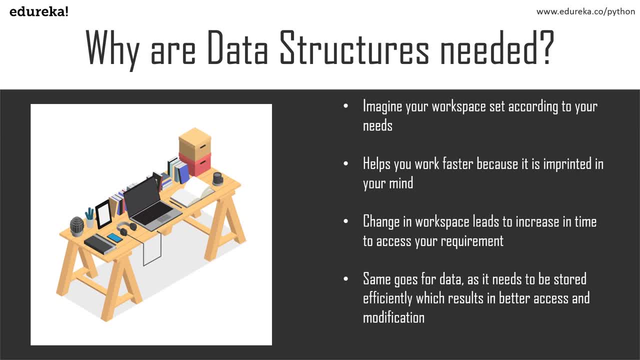 else. you can do that very quickly, even in a crowded setup, as you know what can be accessed from which part of your setup. but what if something is missing or someplace of your device has been changed? it enrages you and you take more time to find out how to get. 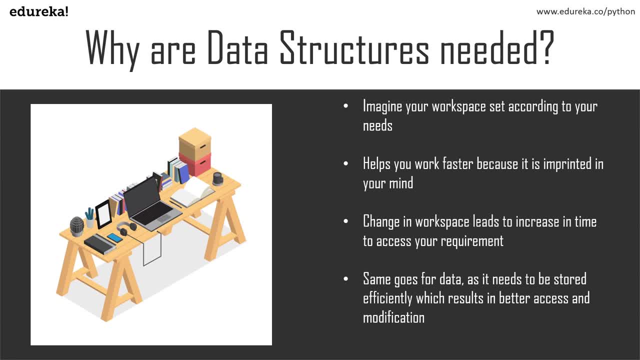 your work done. Now, the worst case- you do not have any setup and all your devices are arranged randomly. It is infuriating when this happens, because you waste time in finding out what you need. the same goes for data on a computer, to it needs to be arranged in a certain manner. 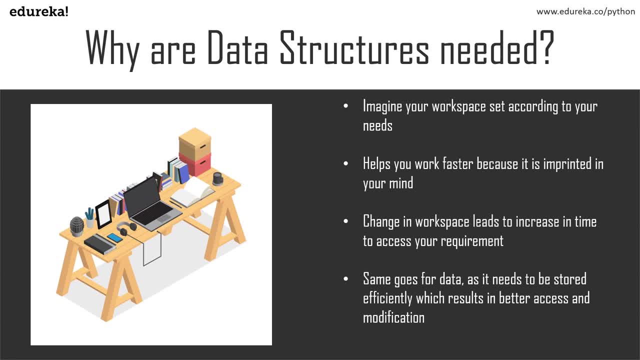 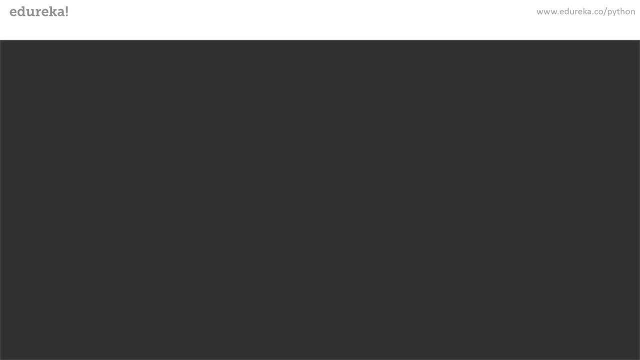 So your computer can access and perform the operations you wanted to. data structures can help us achieve this form of storage and access, and that is the reason they are so important. Now, having understood the importance of a data structure, Why don't we move ahead and 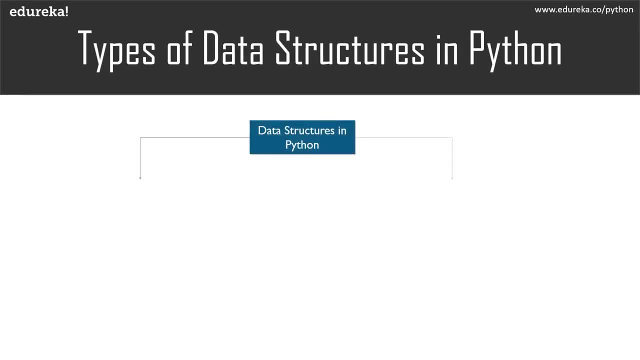 find out the different data structures that python has. python has implicit or built-in support for data Structures that anybody can use, and they also have powerful functions to work with them. the built-in data structures comprise of lists, dictionaries, tuples and sets. on the flip side, python also supports data structures that can be written by users. python supports: 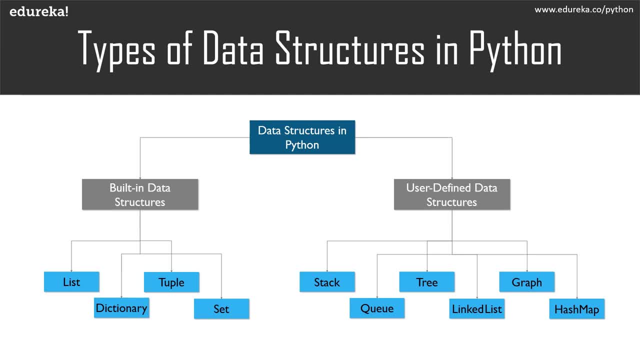 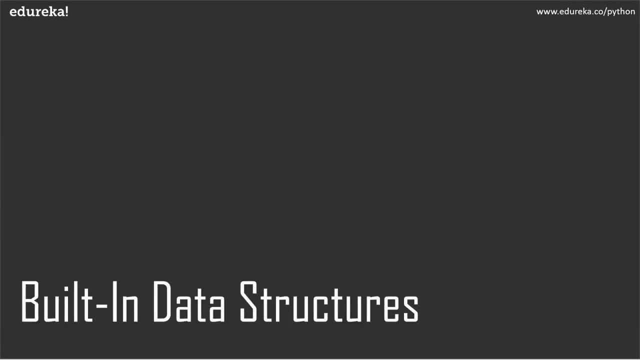 arrays, which can be used to build many data structures. The most common are stack and queue. We have trees, link list, hash maps, graphs. Let's go ahead and discuss each of these data structures one by one. So firstly, let's begin with the 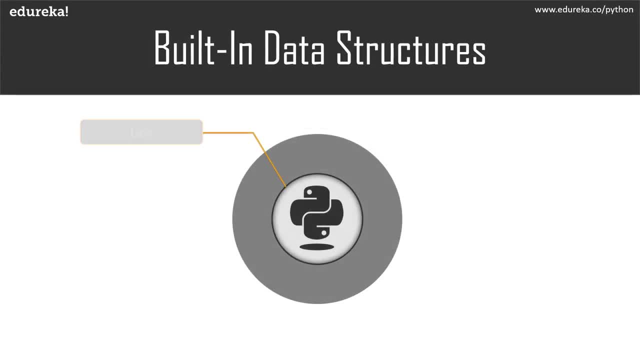 built-in data structures that python has. python has four data structures, which are namely lists, tuples, dictionary and sets. now, for the purpose of the tutorial, I will be using pycharm, So I hope all of you have pycharm installed into your system. So let us go ahead and understand the first data structure, which are lists. lists are basically: 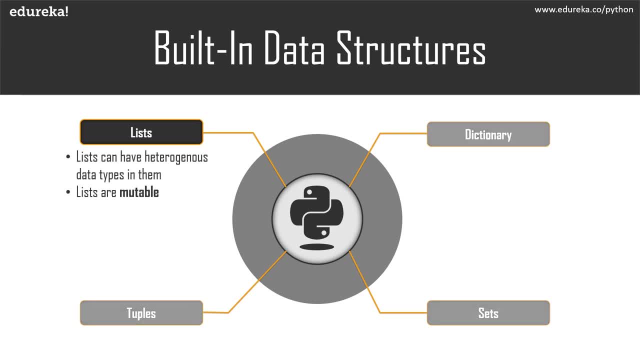 used to store data in a sequential manner, and they can have heterogeneous data types. also in them. lists are mutable, meaning that you can have different types of data and you can even change that data according to how you wanted to. So let's go ahead and execute a program so that you can understand lists much more better. 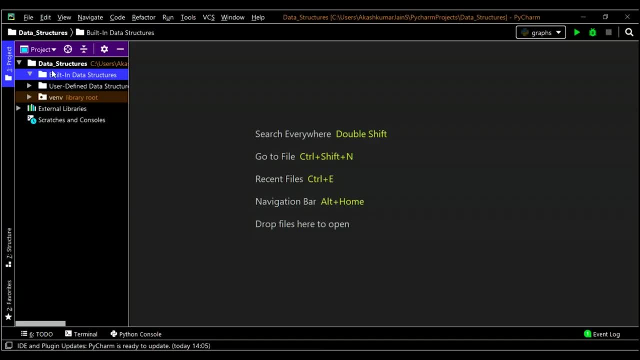 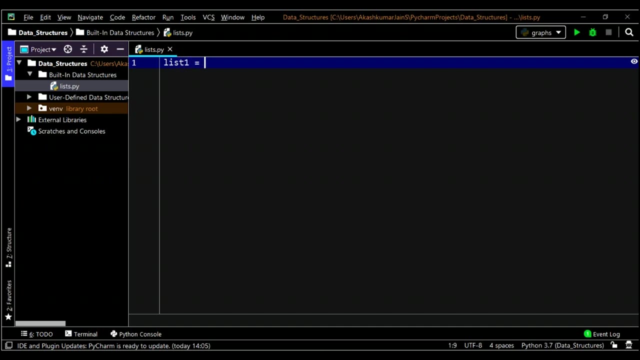 Let me go back to pycharm and let me create a new python file over here. Let me name this as lists enter. So now, how do you create a list? It is basically list. one is equal to square brackets, and that's it. You have created a list over here. 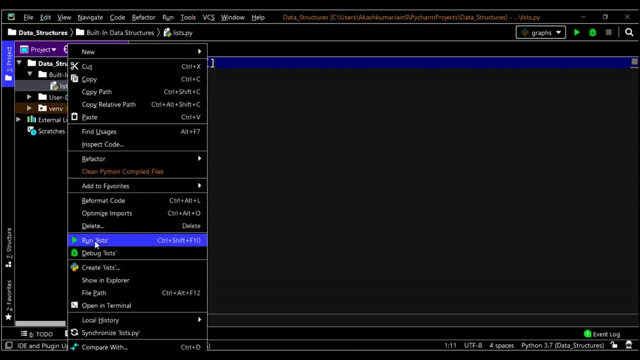 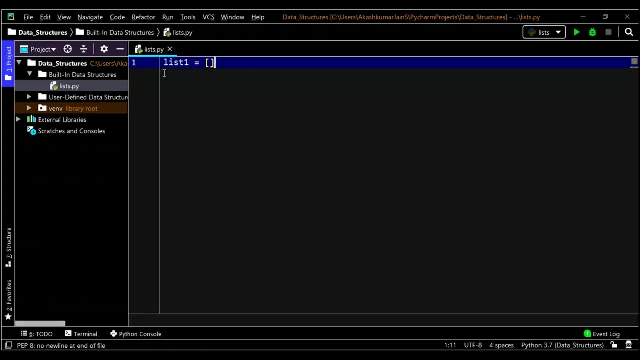 Let me go ahead and run this program for you guys. This right here is an empty list, So let me go ahead and populate some data into this. So let me see it is 1 comma 2 comma 3 and let me just add a string over here so that 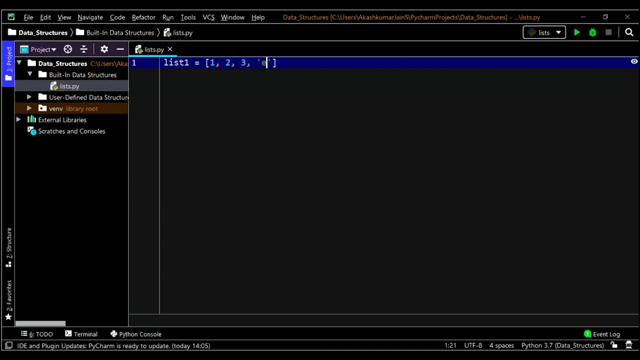 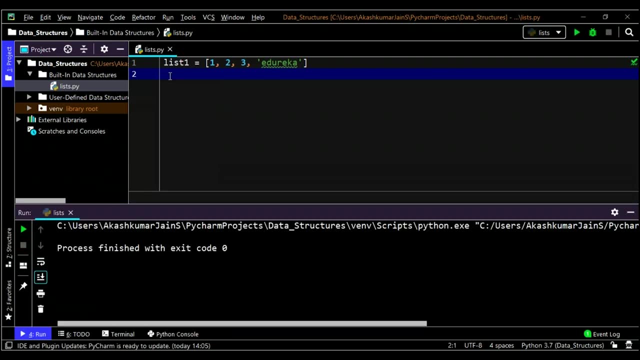 I can show you how you have heterogeneous data types that are supported by lists, and let me run the program again. Sorry, I have not printed anything, So print list one. let me run the program. So, as you can see, this is a list which has 1, 2, 3 and edureka. 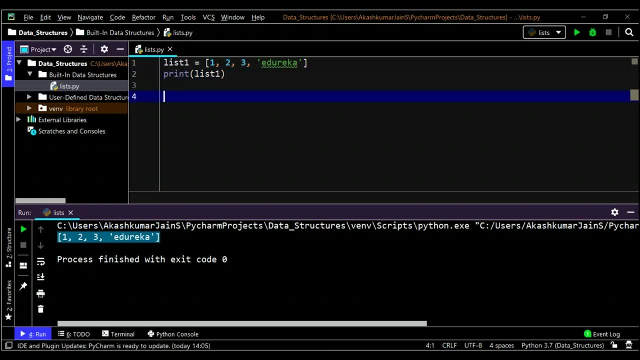 So let's go ahead and learn how to add data elements into this. So we have either the append, we have extend and we have the insert function. These are the three functions that you use So that you can add data elements into your list. 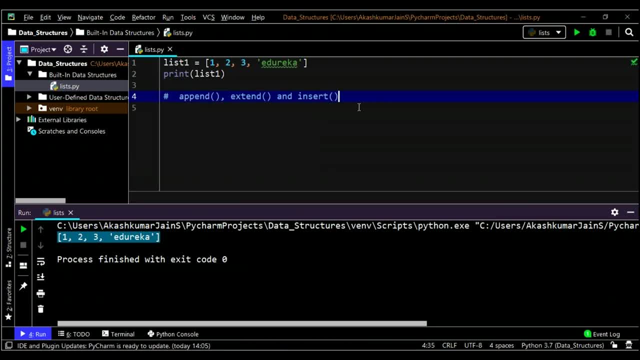 Let's go ahead and add some data into our list. Let's see list one dot append of two. Let me just print list one. Let me go ahead and run the program for you. I'll be removing this print statement so that you do not confuse anything more. 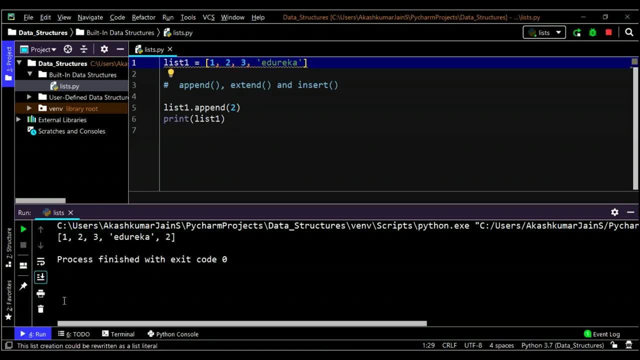 Let me go ahead and run this. So, as you can see, I have 1, 2, 3, edureka and 2. that means 2 has been appended over here. Now let me go ahead and add two elements into this. So if I want to add two elements, I have to make sure that I give it as a single element. 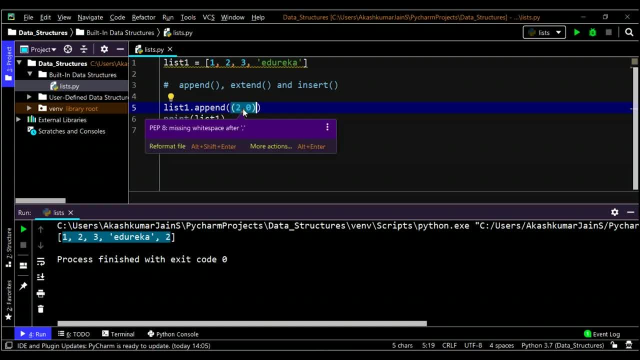 So how do I give this as a single element? I give it using the parenthesis or square brackets, anything that you want to. so, basically, you are trying to give another data type into the append function. So let me go ahead and run the program. As you can see, 2 and 0 has been added. now let me go ahead and use the extend function. 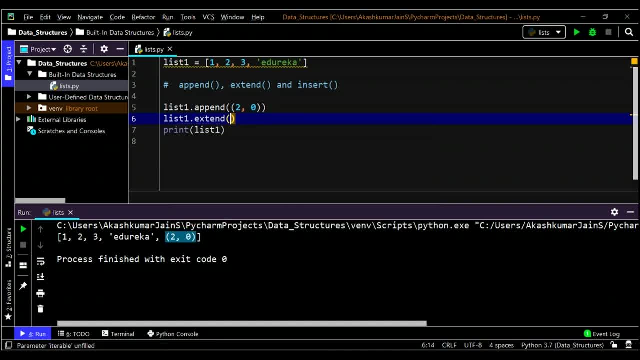 list one dot extend, and let me give the same values, 2 and 0, and let me run this again So you can see the difference. what append and extend functions have? we have 1, 2, 3, edureka, which was already present, and then we have 2- 0. 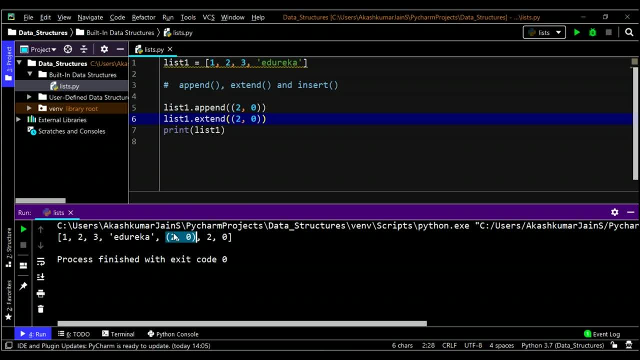 Which has been added as a couple will understand more about couples later in the video, but just know that anything in a parenthesis is a couple. and then we have 2: 0, which is basically single elements over here, and this is a couple. so that is the difference between the append. 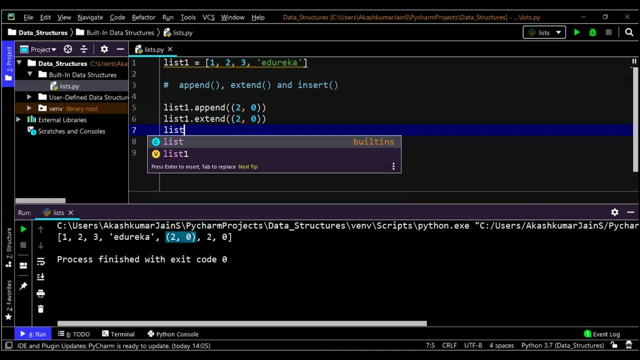 and the extend function. Let us go ahead and write the insert function, So we have insert, and then I give the index over here. So I want it at the third position. Let me give the element Add As example. let me run the program again. 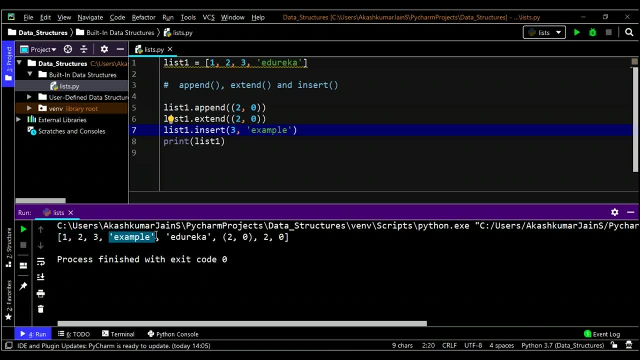 So, as you can see, 1, 2, 3 and example was put in the index of third position. So I hope all of you understand what indexes are. if you do not know what indexes are, Let me just tell that to you. So, basically, indexes are addresses in which you can access the data which you have stored. 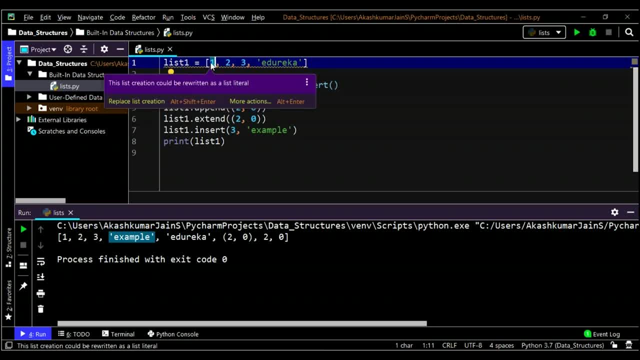 So the first element of the list is always having the index 0. And then this element has the index 1, this element has an index to this element as an index 3, and so on for how many ever elements I add. So that is basically what happens over here. 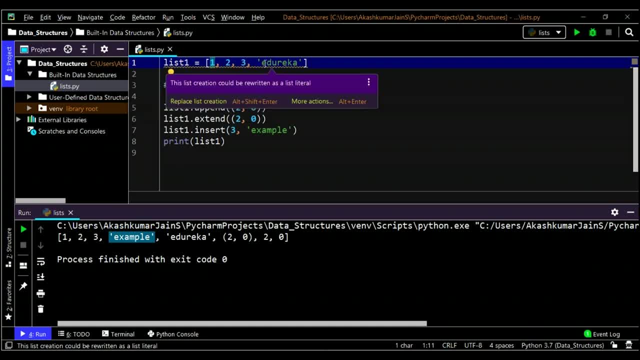 This will be index 0, index 1, index 2 and index 3.. I can also have elements from the backside of the data, So edureka will have minus 1.. So basically, I can even access elements in the reverse order. 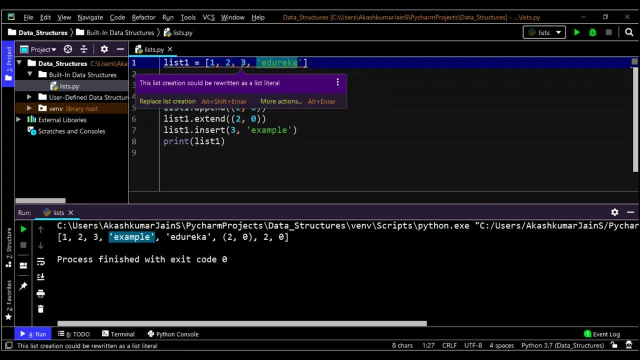 So edureka will have the index as minus 1.. This will be minus 1.. This will be minus 2, minus 3 and minus 4.. So I hope you've understood what basically is used to append data into it. Let me go ahead and show you how to delete data. 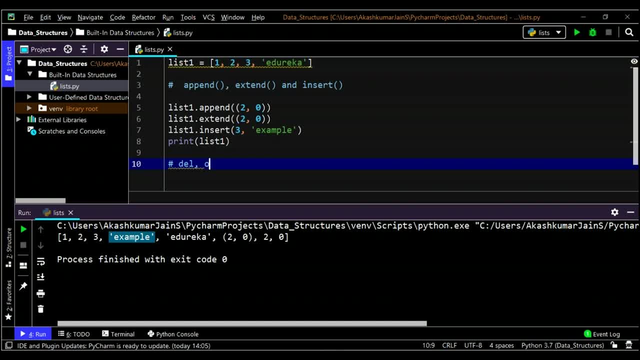 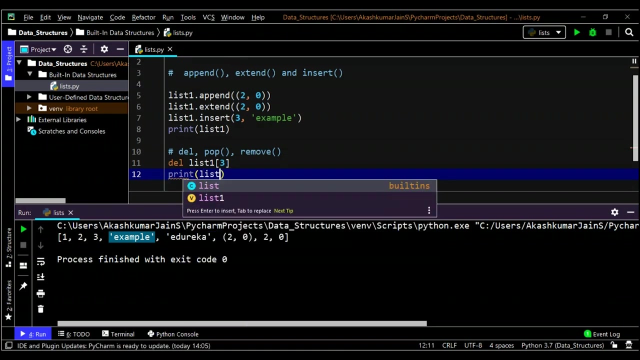 So we use the del keyword, then we also use the pop function And we also use the remove function. Let me just do delete of list one, of let's say what element I want to remove example. So let me just give three. Let me print it over here now. 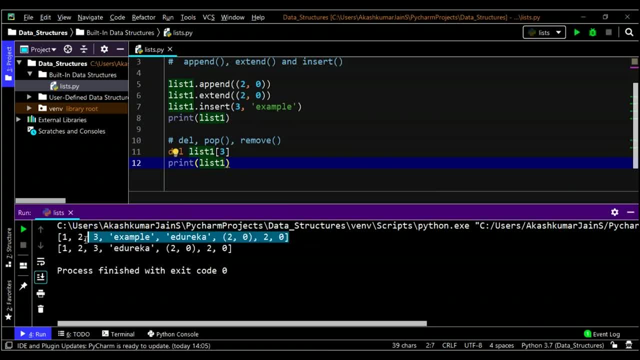 Let me run the program again. So, as you can see, there was example here and I have deleted example over here. Now let's do the next one, which is the pop function list. one dot pop, and let's say that I wanted to move 0, 1, 2, 3 and 4, so 4.. 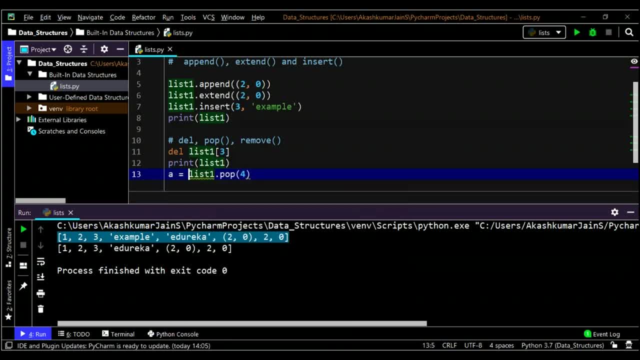 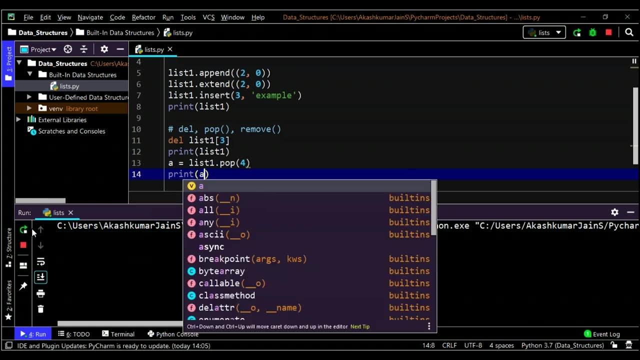 And I can even print this: equal to, because pop function basically gives back the data that has been deleted. The del keyword does not do that, So let me just print a, let me run the program So as you can see over here that the element of a has been removed. 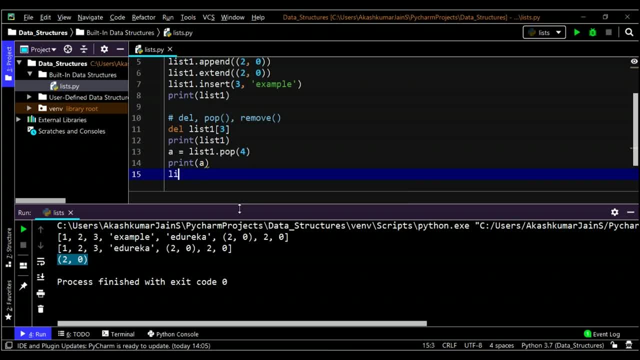 Let's remove data using list one: dot remove. Let's delete two. Let me run this program. So you have to print this. print list one. So the first two has been deleted over here. So that is basically how you delete elements, As you can see over here. 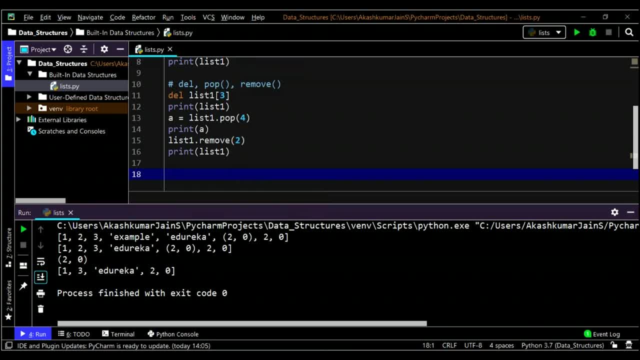 We have really good functions which are used to add elements, delete elements. How do you access the elements? It's really simple over here. Let me just show that you just do the print one. if you want to access particular elements, you can do list one of. let's see. if you do not give any start and stop indexes, it will. 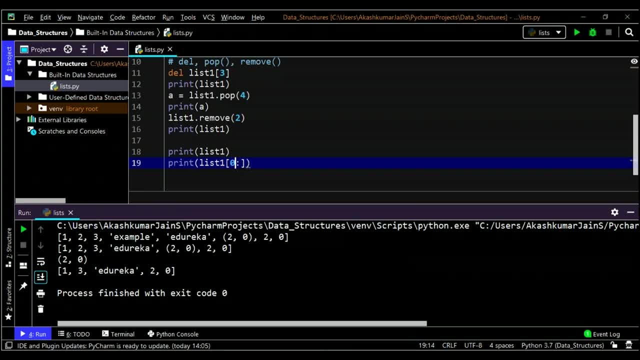 print the whole list. Let me just say that this is from 0 to 2. then if I want to skip elements, I can just do the list one of 0 to 4 and skipping two elements if I want to print it in the reverse order. 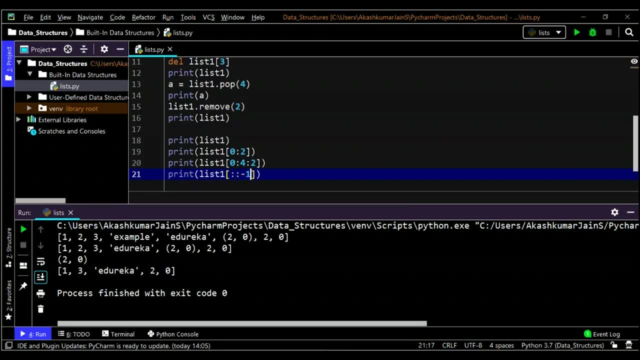 I can just do list one And minus 1. let me go ahead and run the program. Yes, as you can see, I have 1 comma 3 at Eureka to 0, then I have 0 to 2. 0 and 1 will be printed. 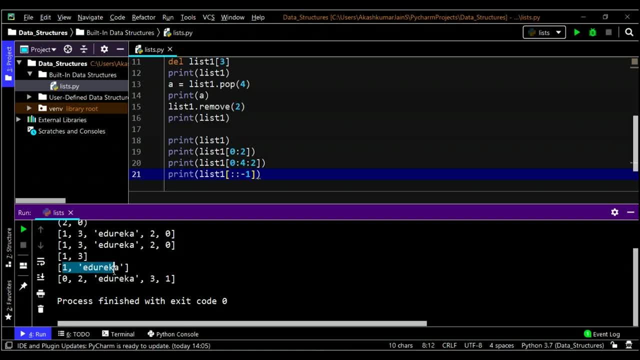 and 2 will be rejected. then I have 0 to 4 and I am skipping it in steps of 2, and then I have the list one which is reverse order. So I have 1, 3 at Eureka, 0 and 2 in the reverse order. 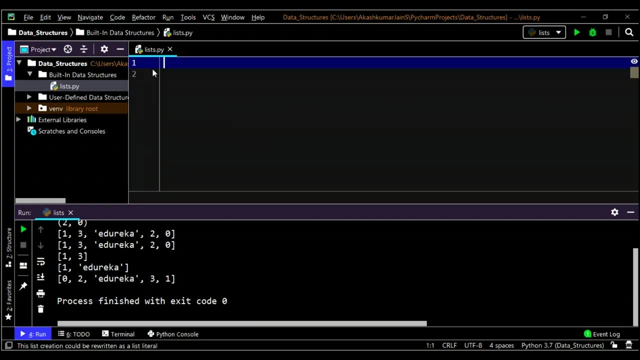 Let me clear All this up. I hope you've understood all of this, because I'll be adding a new function which will require data of same elements to be there. So let me just say list one of 1 comma, 2 comma, 3 comma, 65 comma, 1, 2 comma, 5, 46, 0. so I have. 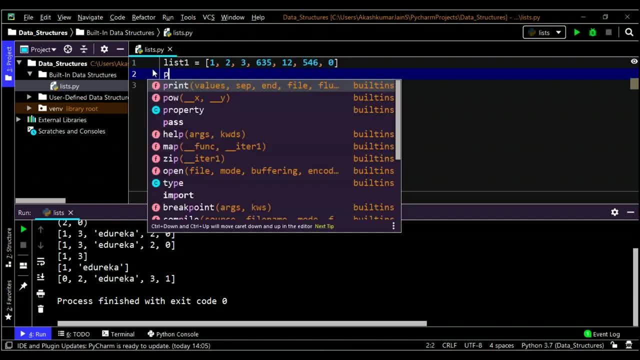 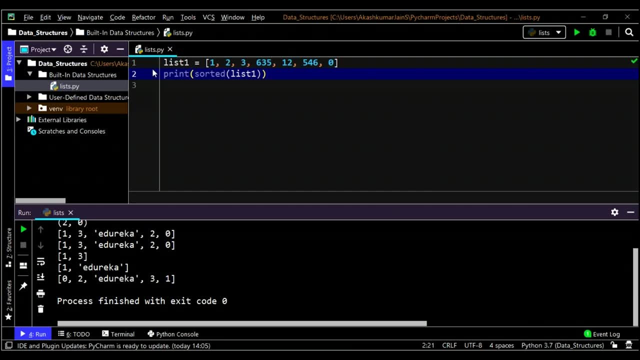 two methods over here which are sort and sorted. So let me just show what sorted does. So let me write Sorted of list one. Let me run this So, as you can see, the output is giving me a data in the ascending order, but the actual 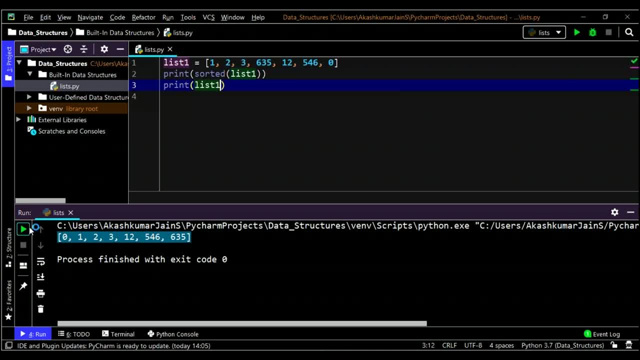 list data has not been changed, So let me print this again. Yes, So as you can see, the original data of the list has not been changed. If I actually want to change the original data list, I would have to use the sort function. 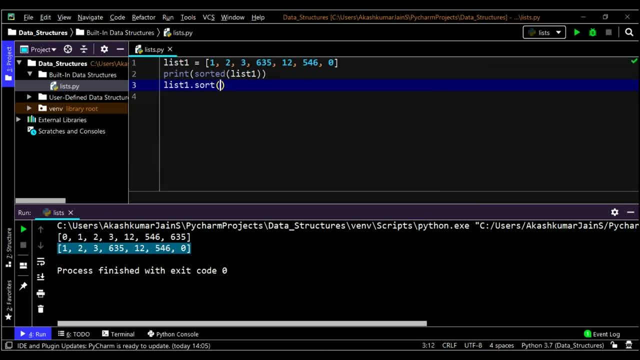 So I do the list one, dot sort. So that means, if I want to sort it in the descending order, doing the reverse is equal to true and let me just print the list one. Let me run the program So, as you can see, data has been sorted in the reverse order. 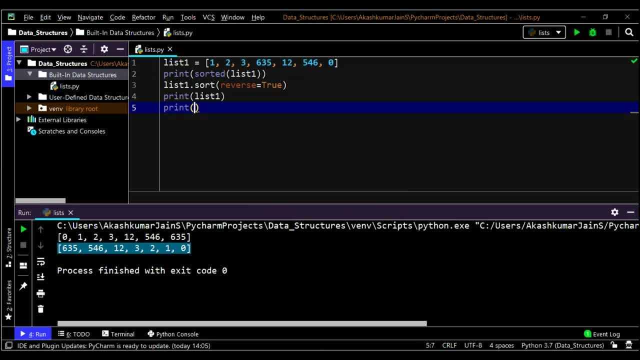 We have another function which is used to find out the index of a particular element. So let us go ahead and find that out. So let's just see that this is list one, dot index of two. Let's go ahead and print this, As you can see that this is at value zero. 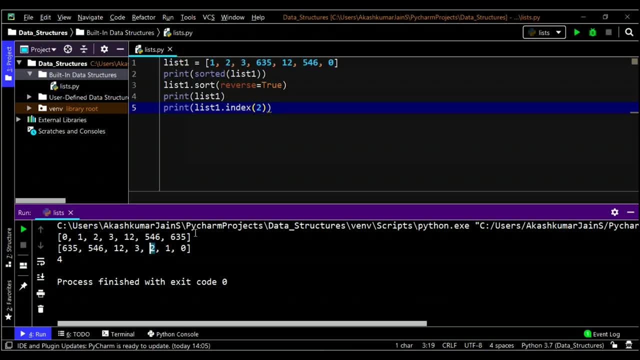 This is at value 1, 2, 3 and 4, and that's the reason we have obtained the value as 4.. Let's go ahead and find the count of a particular value. So it is list one dot count of 12.. 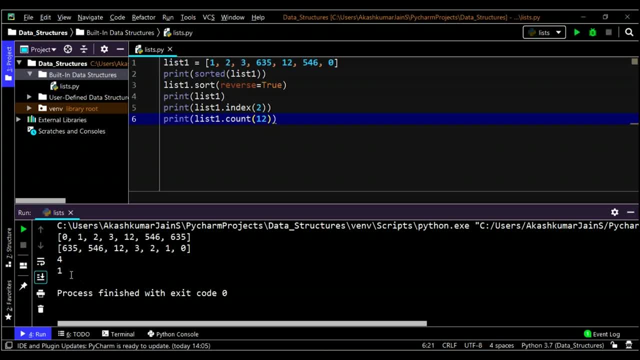 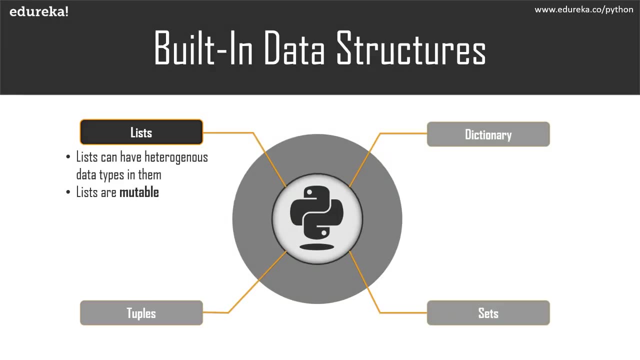 Let me go ahead and run the program. So it is saying that 12 has been occurring once in the list. So that basically wraps up The functions of list. I hope you've understood it much more clearly. Let me go ahead and delete the program. 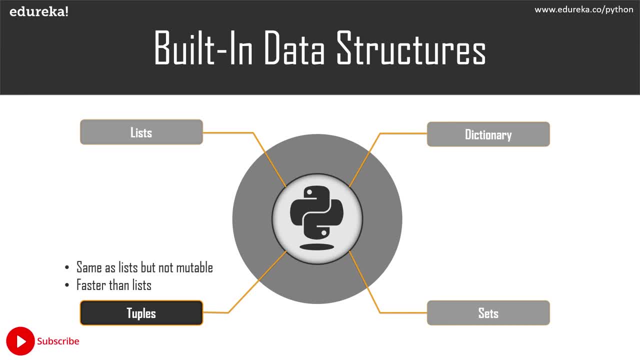 What are tuples? tuples are basically the same as lists. The only difference is that they have parenthesis and they are not mutable, meaning that you cannot change the data in the list. So let's go ahead and write a program for that. So let me just call this as tuple. 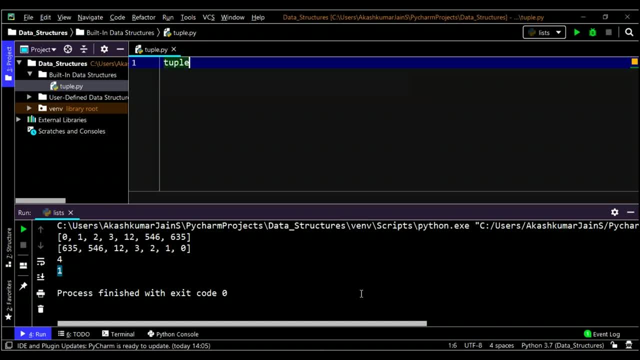 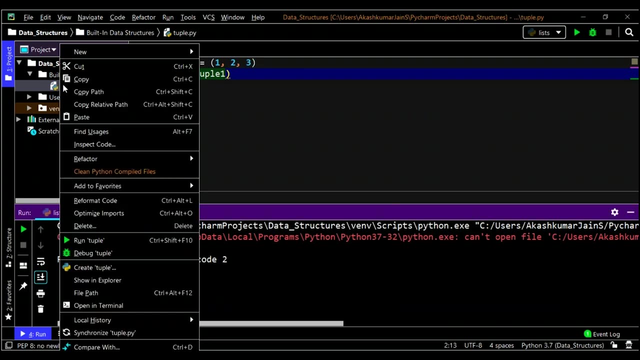 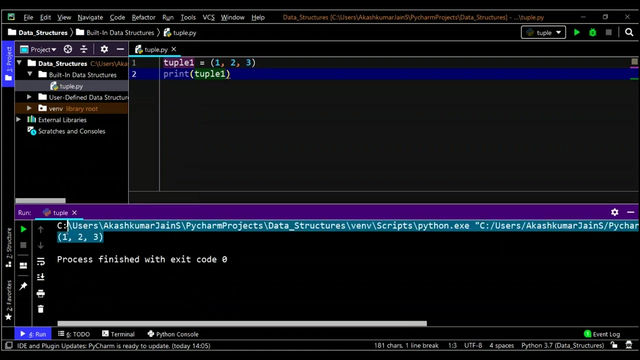 Now let me write a tuple over here. So I have: tuple 1 is equal to 1 comma, 2 comma 3.. Let's go ahead and print this tuple. So let's just write tuple 1.. Sorry, so as you can see, we have 1, 2, 3 and then it's basically the same functions. 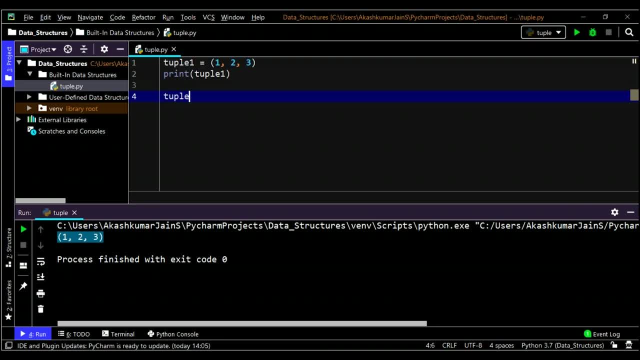 So how do you add data into the tuple? you do that using concatenation. So tuple 1 is equal to tuple 1 plus adding another tuple. So let's just say this as 4 comma, 5 comma 6.. Let me print tuple 1.. 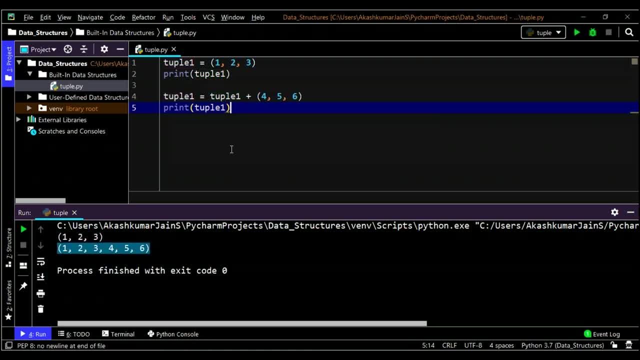 As you can see, it is 1, 2, 3, 4, 5, 6.. Now, if I want to change any data in my tuple, I am not able to do that. Let's just check that out. So let me just say there: 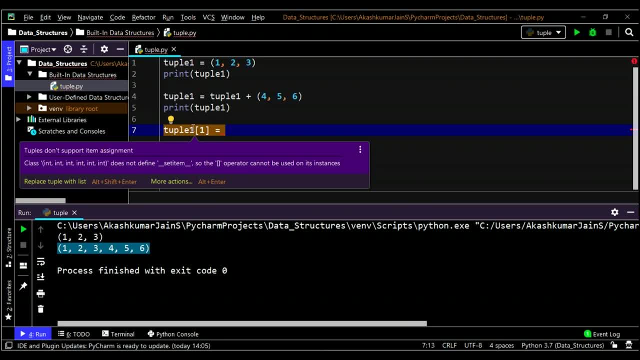 1. Is equal to, and you can see it is already giving me a warning saying that tuples do not support item assignment, So I cannot change data in the tuples, Whereas this would have been legal in a list. Let me show you the difference. 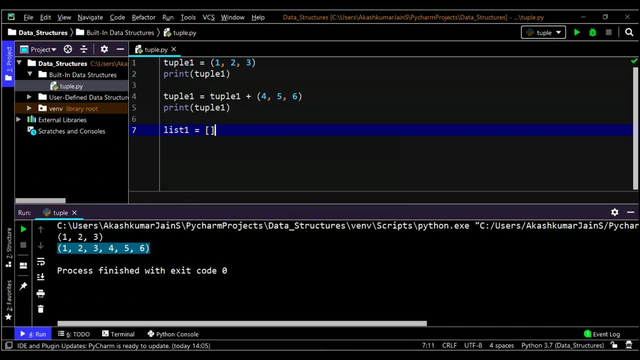 So if I had a list, say list 1 is equal to 1, comma, 2, comma 3, and I want to change list 1 of 1 is equal to 5, and if I print List 1.. As you can see, I have declared 1, 2, 3 over here. 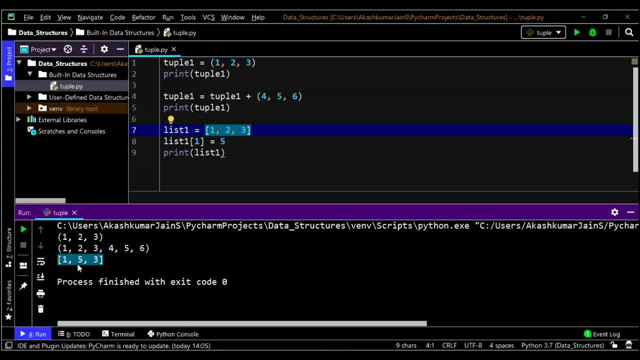 and I have changed the value over here, but that is the reason I am getting 1 5, 3 over here instead of 1 2, 3.. So this is allowed in lists. part changing data in the tuples is not allowed. So you access tuples the same way as you do it for lists. 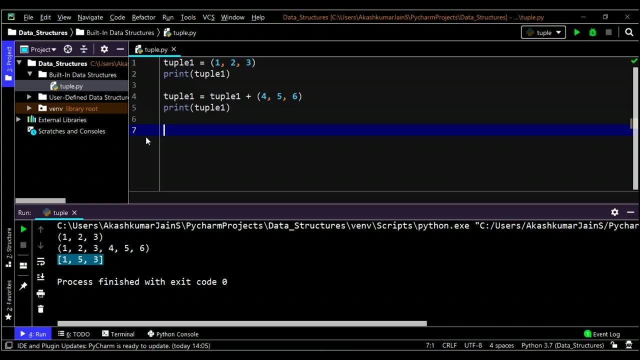 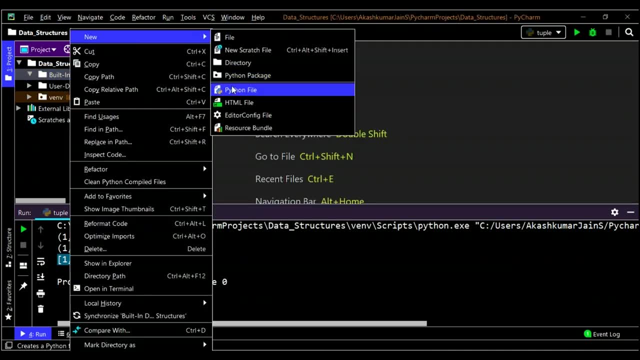 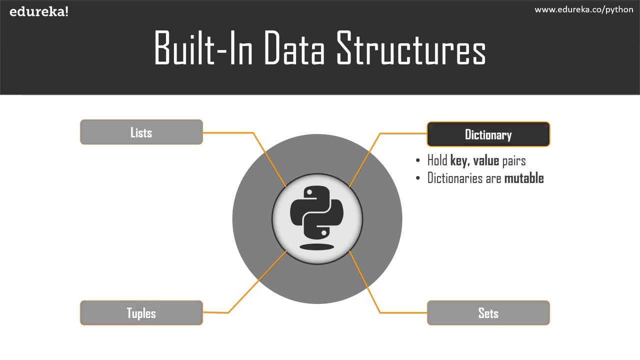 and all the rest is the same as lists. So that's basically wrapping up our tuples. Let me go ahead and open. dictionary Is for you guys. So what is a dictionary? dictionary is basically: or data structure that holds key value pair. So what do you mean by a key value pair? 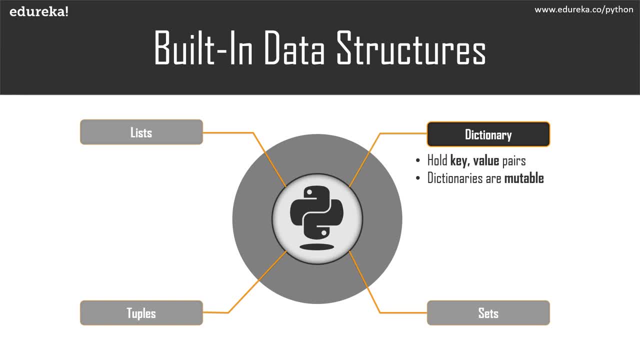 So you have something as a key or something which is common and you have a value for it. For example, if you have your name or the names that are stored in a company, they may have one particular first name or last name. Those are basically keys. 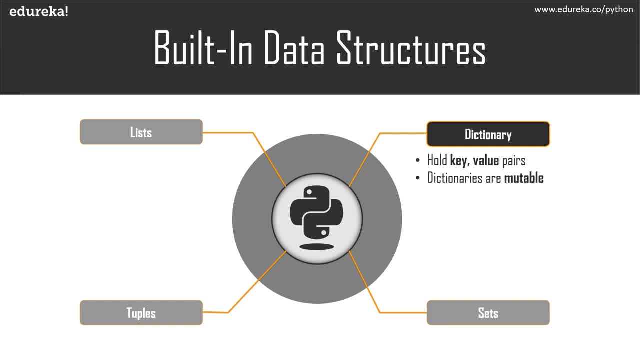 and the values that you enter for those that are basically key value pairs. So what is a key value pair? A key value pair is basically a key and a particular value for it. A key may be something like the first name or the last name in a company. 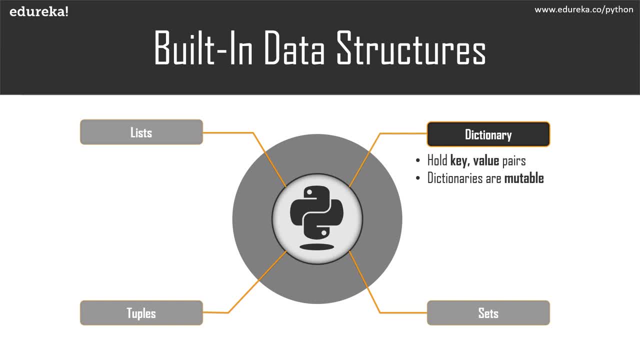 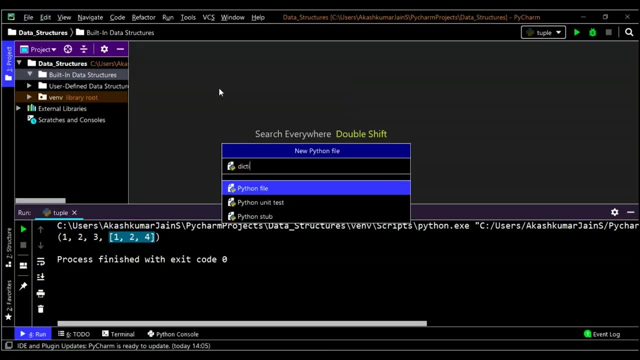 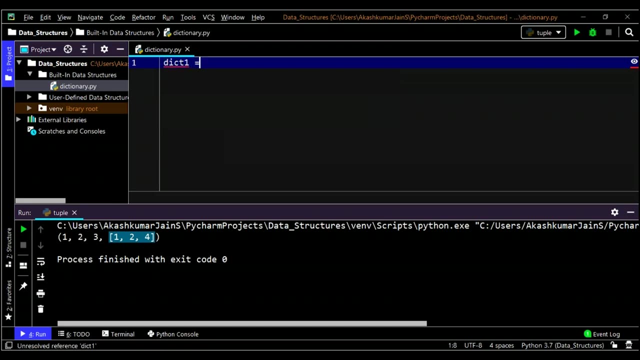 and the other names that you enter for those. Those are the values. Let's go ahead and write some programs for dictionaries. Let me go ahead and create a new File over here. Yes, So how do you create a dictionary? It is a dict. one is equal to one as. 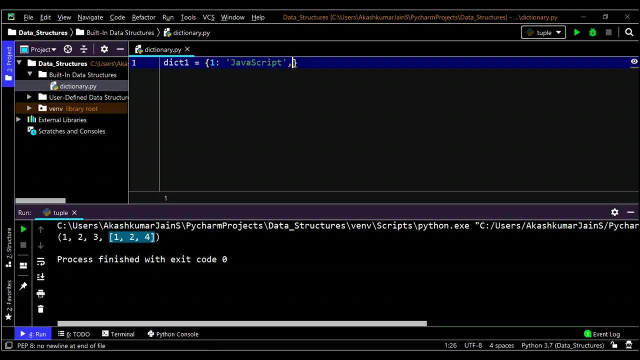 Java script, Comma 2 as Java, Let me go ahead and print dict one. So, as you can see, one is the key over here and JavaScript is the value. 2 is the key and Java is the value. So that is basically how you write your dictionary. 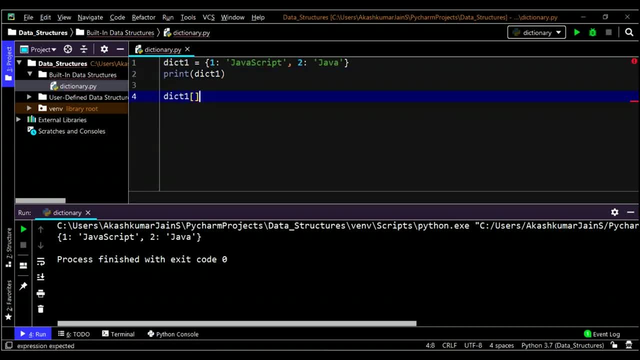 Let's change values inside the dictionary. It is a dict. One of one is equal to Python. Let me go ahead and print in dictionary one. Let me run the program So, as you can see, JavaScript is now changed with value Python. that is basically how you can change values inside. 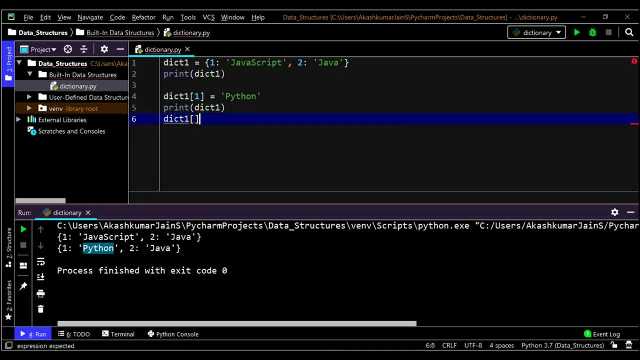 How do you add values? So we add values. giving a new key value pairs You. for example, let's write 3 is equal to Ruby print Nick one. As you can see, I have added a new value. So that's how simple it is to work with dictionary. 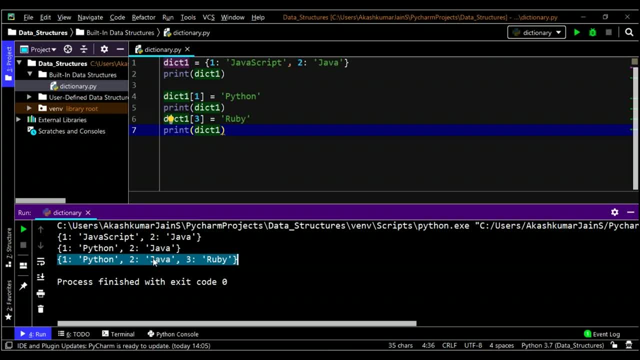 So we have learned how to write a dictionary, How we can change the values in a dictionary, how to add values into a dictionary. Let's go ahead and learn how to delete values for deletion. It's the same. we can use the del keyword. 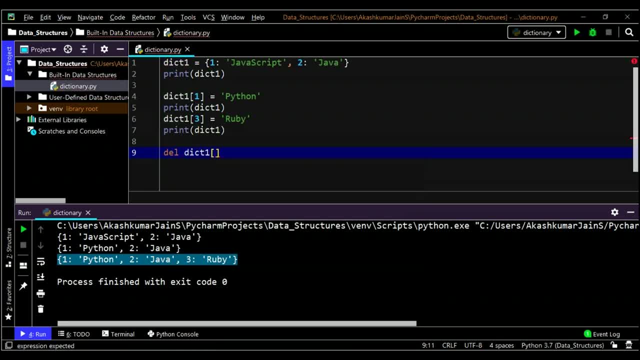 So let's say it is del dict one of one. What is value one will be deleted. So whatever is the key where one is the value, So python has the value one, This will be deleted. Let me just show that to you. 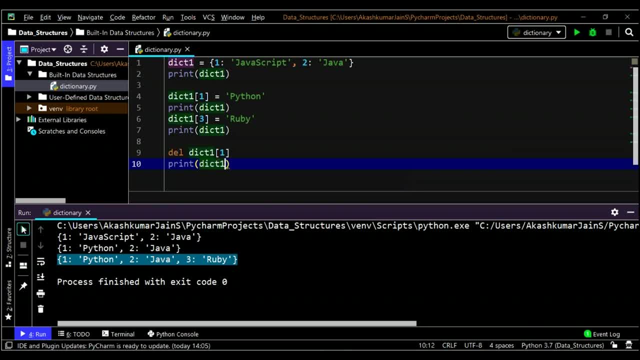 So we have print dict one, As you can see, key value pair of one and python is deleted. So that's how you do it. Let me show you another method, that is, the using the pop method. It is a dict one of pop and I am popping the key value pair. 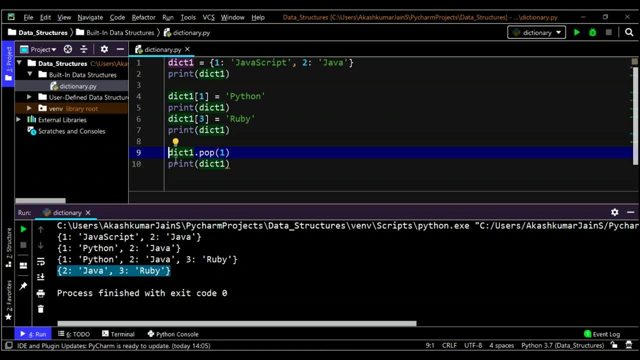 which has the key one, and I can even print this, Because pop has a return value. Yes, So, as you can see, python was popped out and two and Java has been remaining in the dictionary. I have another thing which is called as the pop item. 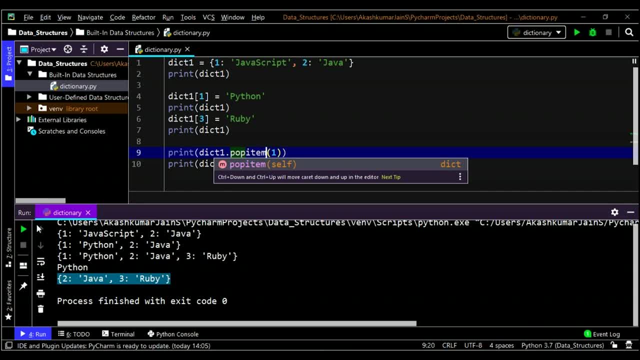 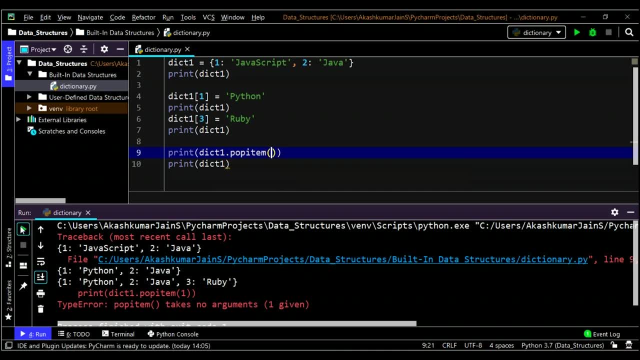 and this will return a tuple with the key value pair. Let me run the program. Oh sorry, I cannot give any arguments to pop item, So let me run this again. So, as you can see, three and Ruby the value which is in the end. 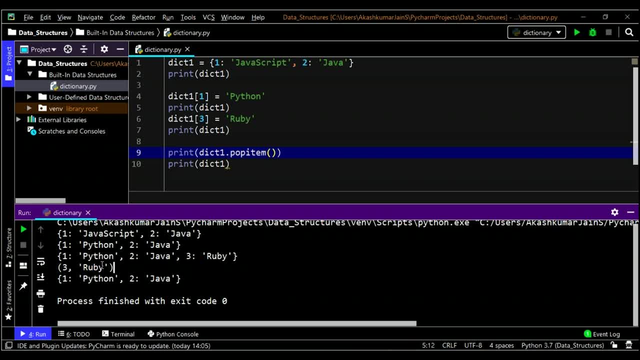 will always be popped using the pop item. So three and Ruby has been returned as our tuple One, python and two and Java remaining in the dictionary. We have a bit of more functions. Let me just show those to you. So we have dict. one dot keys is to get all the keys. 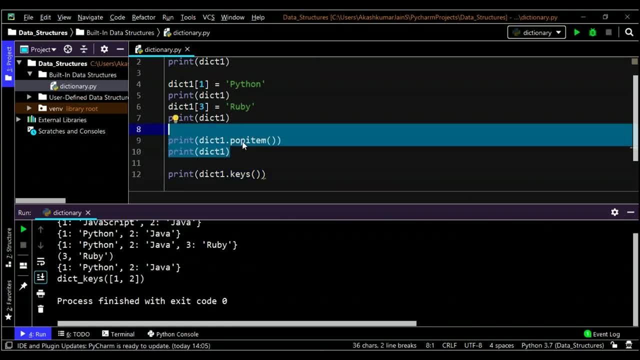 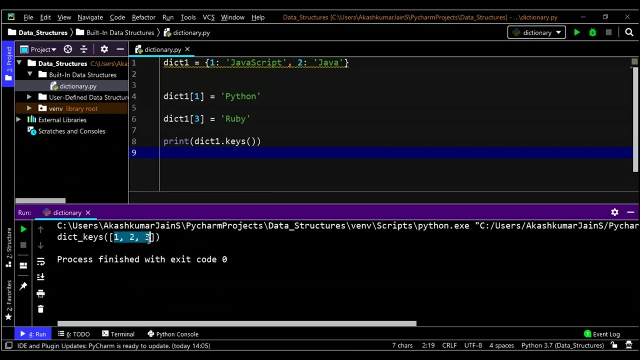 Let me print that for you. Let me remove all of these redundant prints So that I can just show you all the keys that are required. Let me print all the keys. So the keys are 1, 2, 3. if I want the values, I have the values. 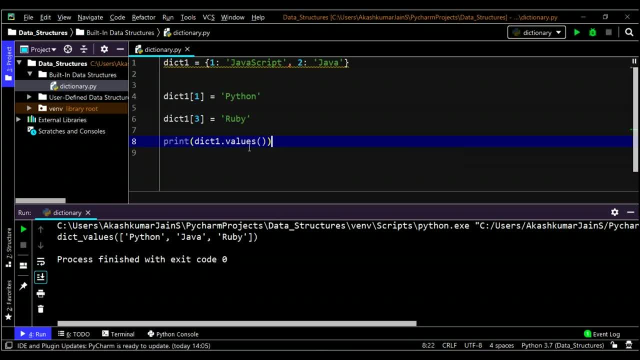 So this should be python, Java and Ruby, and if I want the items, which is the key value pair, I just write items. So, as you can see, I have one python 2, Java 3 and Ruby which are returned as the key value pairs. 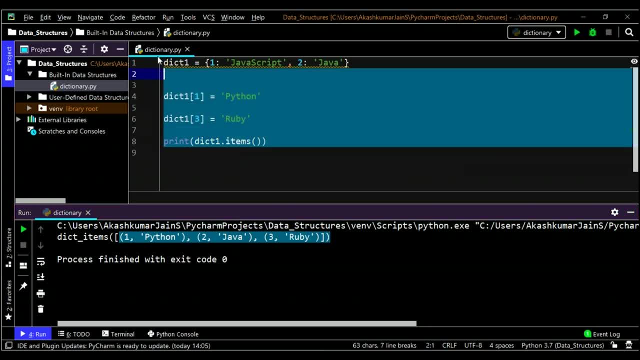 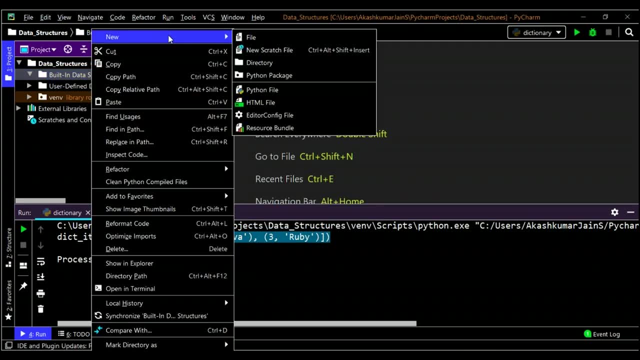 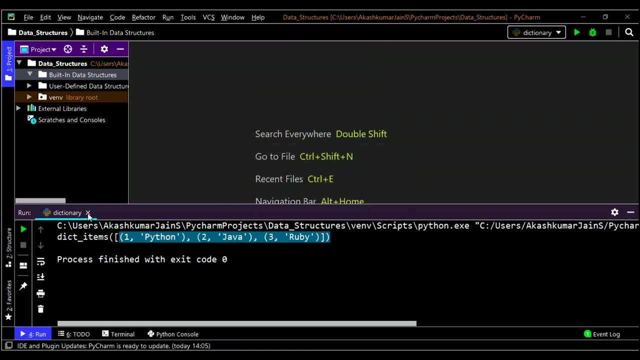 So that is basically what wraps up our session for dictionaries. Let's move ahead with sets. So let me name this assets. So if you are familiar with how a set works in arithmetic, it is really easy for you to understand what sets are in python. 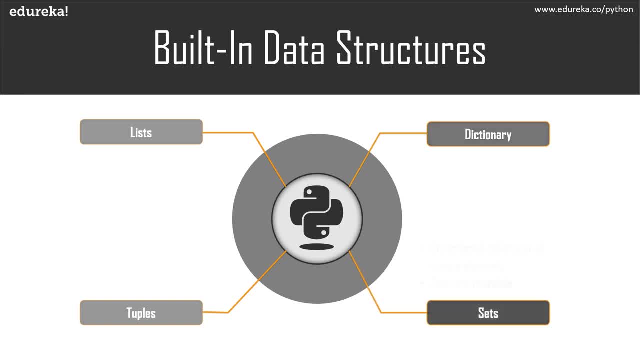 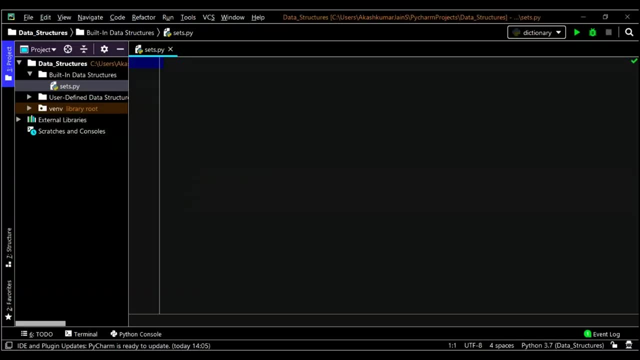 So let me go back to the presentation. So, as you can see, sets are an unordered collection of unique elements and they are mutable. So let me show that to you. So set one: you have to remember that if you do not add a key value pair, it is always taken as a set. 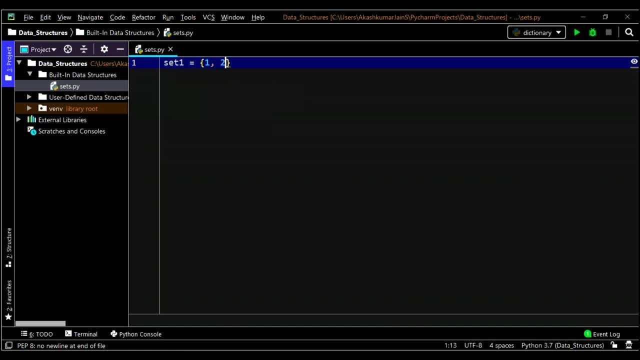 But if you add a key value pair, it is always a dictionary. Let's see: This is 1 comma, 2 comma, 3 comma, 4, 4 and 4.. Let me print set one. Now you will understand what a set is basically. 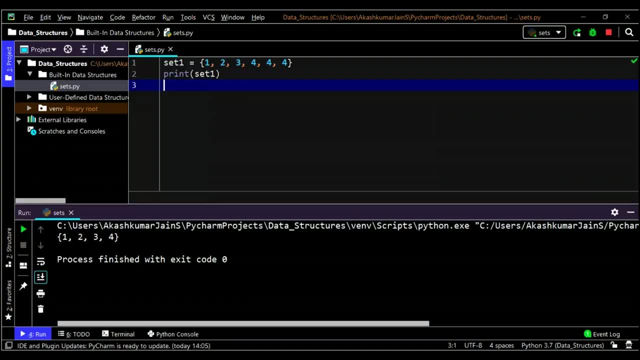 because I have repeated for thrice, but as you can see in the output it is only taken it as once. So that is basically what the set is. Let me go ahead and show you how to add elements. So you have set one dot, add of five. 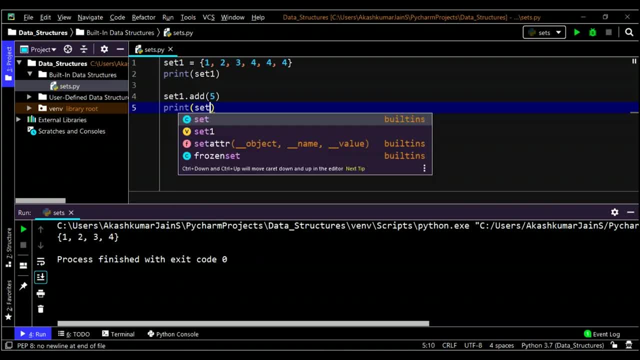 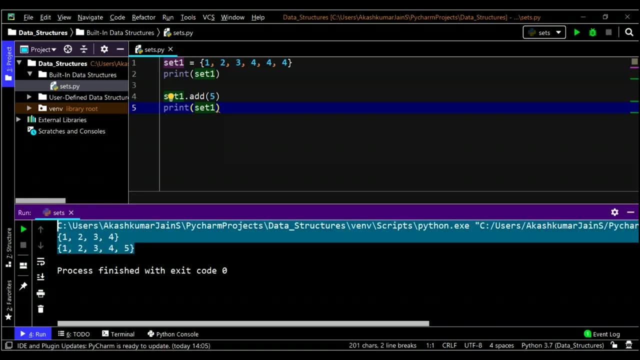 Let me go ahead and print this. Yes, So, as you can see, 1, 2, 3, 4, 5 has been added. That's how simple it is to work with sets. So let us go ahead and now understand What are the different operations that sets have. so it has Union. 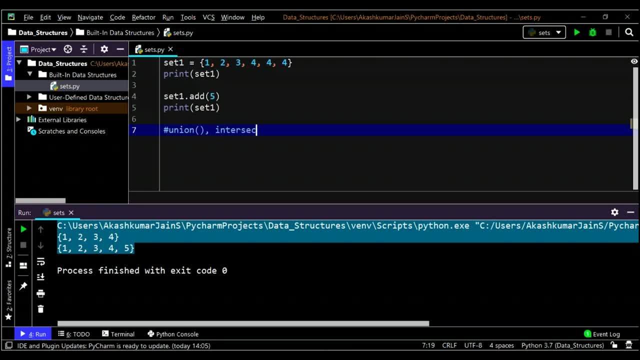 Let me just comment all of it. It has the intersection, It has difference and it has symmetric, Symmetric difference. So these are the four functions that are available to us. So let me go ahead and write another set, because we need two sets for working with this. 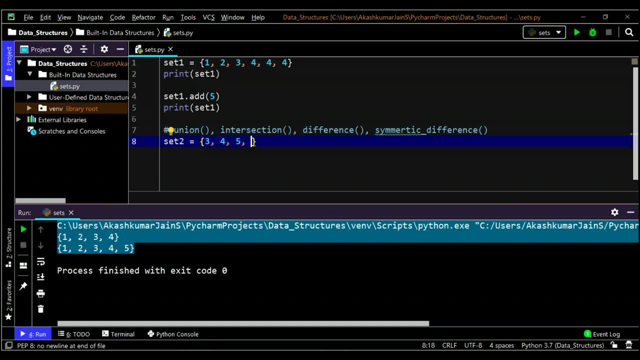 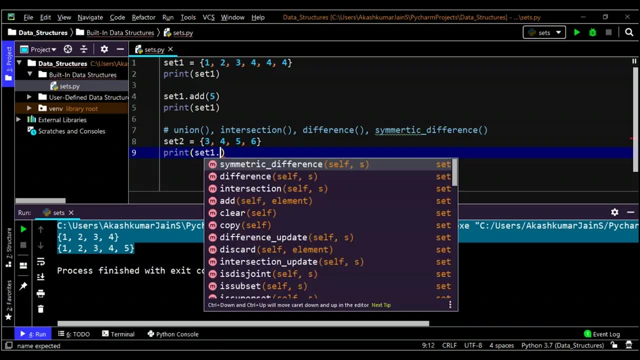 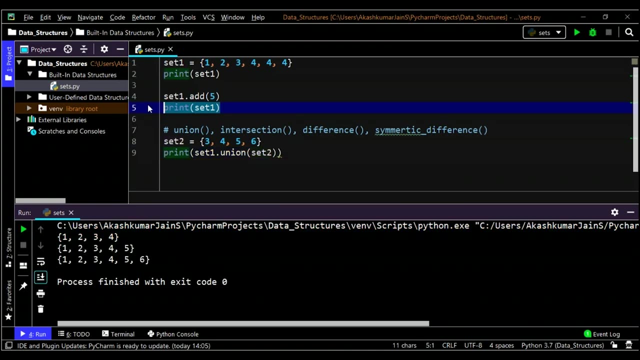 This will be 3 comma, 4 comma, 5, comma 6.. So let me just say: print Set 1 dot, Union of set 2.. Let me go ahead and print this. Firstly, let me remove these redundant statements, So let me run the program now. 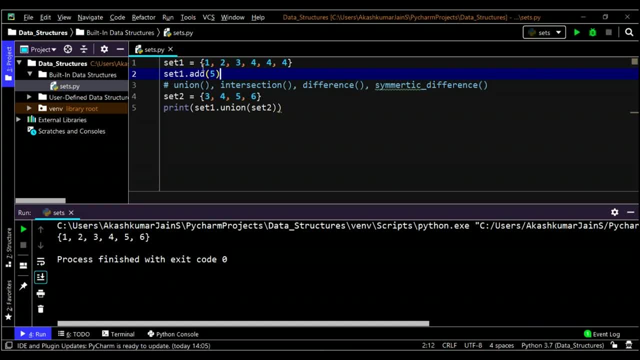 As you can see, 1, 2, 3, 4, 5, 6 is the Union, because we have 1, 2, 3, 4 in set 1 and 3, 4, 5, 6 in set 2.. So whatever is common in both of those, 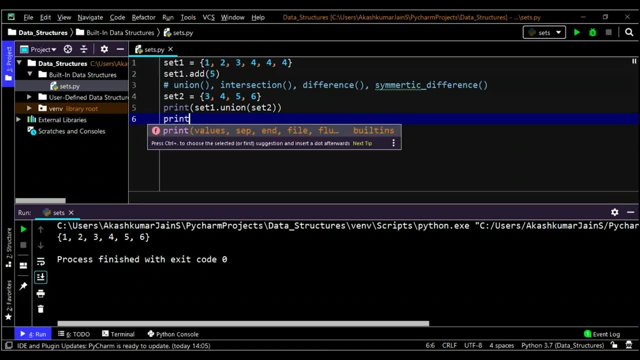 Will be added and given out as a list. Let me print the intersection of this. So it is set 1 dot. Intersection of set to. let me run the value. So what is common? it has 3, 4 and 5, because we had added 5 over here. 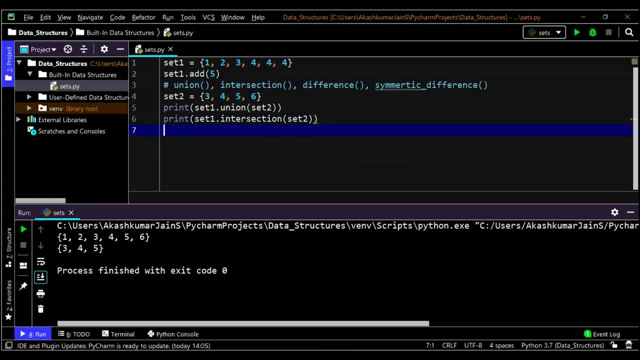 So we have 3, 4, 5, which is the intersection, which is the common elements in both of them. So let's go ahead and find What is the difference? we have Set 1 dot. difference of set to what this does is basically whatever is common in both of them will. 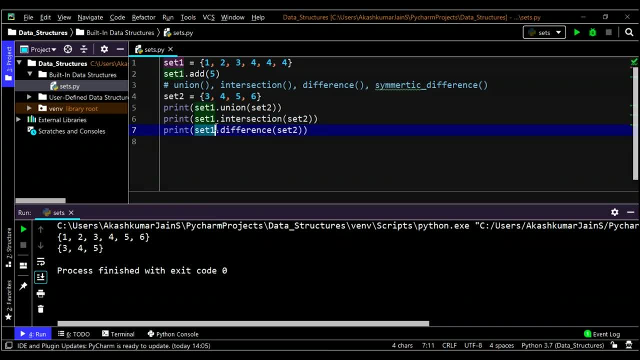 be taken out and whatever is remaining in set 1 will be given as the output. So it should be 1 and 2 right now, because 3, 4 and 5 are common. So 1 and 2 has been given as the output to us. 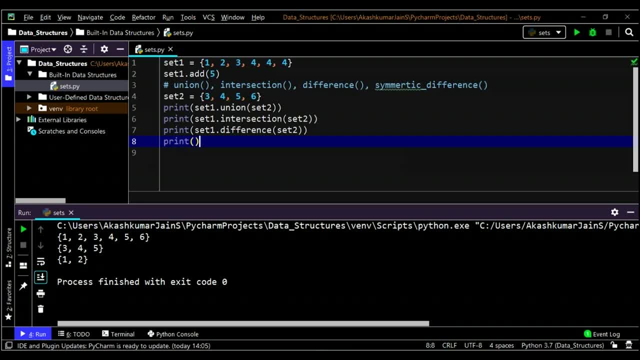 Now, what is symmetric difference? symmetric difference is the same as difference, with the one change that both the elements of Sets will be given as the output. whatever is common in both The sets will be taken out and whatever is remaining, both The sets, will be given as the output, that is, 1, 2 and 6.. 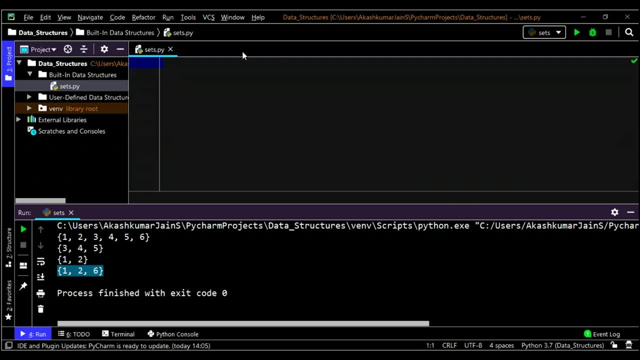 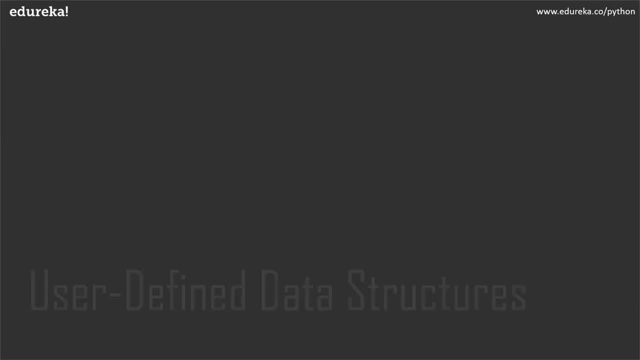 So I hope you're clear with how sets work. and that basically wraps up all of our inbuilt data structures that we have with python. So now that we have finished all the inbuilt data structures, let's move ahead to the user-defined data structures that python has. 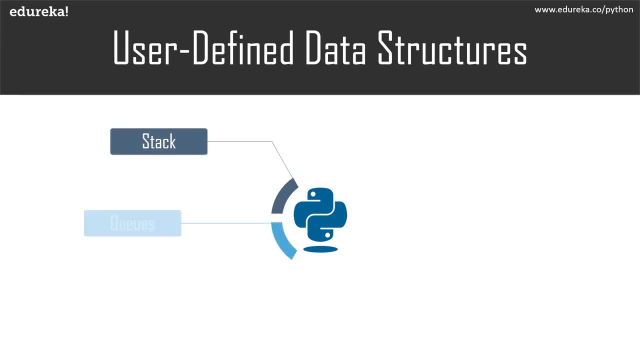 So, as you can see, these are the different data Such as that python supports. we have stacks, queues, trees, hash maps, You have graphs and linked list. So you would want to know that we will not be doing a tutorial for hash map, because hash map is basically what dictionary is. 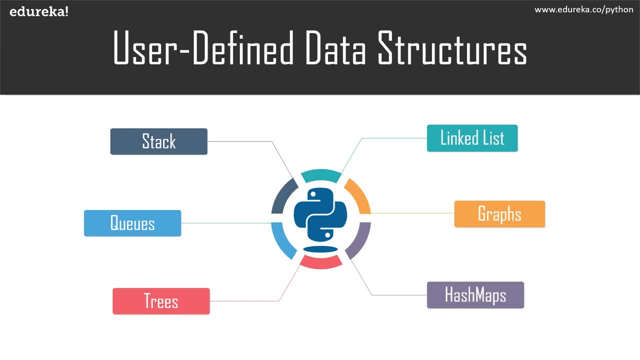 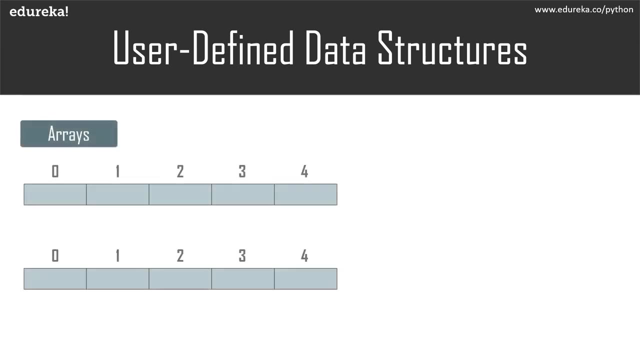 So repeating hash map and dictionary is of no use and basically they have the same application and that's the reason I won't be showing your demo for that. So we will be doing a demo for a stack queue, trees, linked list and crafts. Let's move ahead and understand each of these one by one now before starting out. 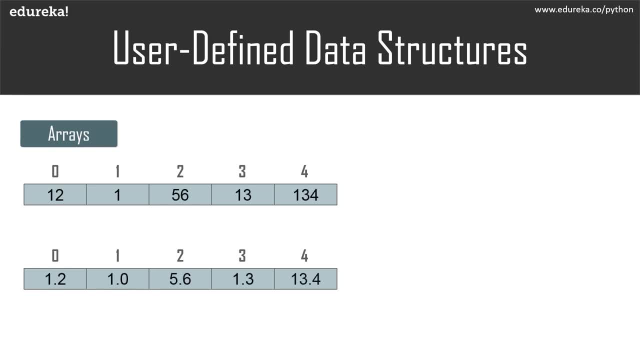 We would firstly need to know what an array is. If you remember what a list was, that is basically what an array is. The only difference is that arrays have only one data type. That means if it is a data type of integers, only integer data type will be taken. 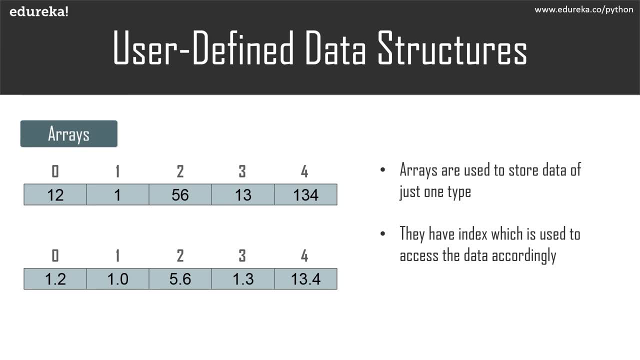 if it is a floating number, only floating data types will be taken into the array. So that is what is The only difference between an array and a list. So arrays are what are basically used to. you know, create your particular data structures. 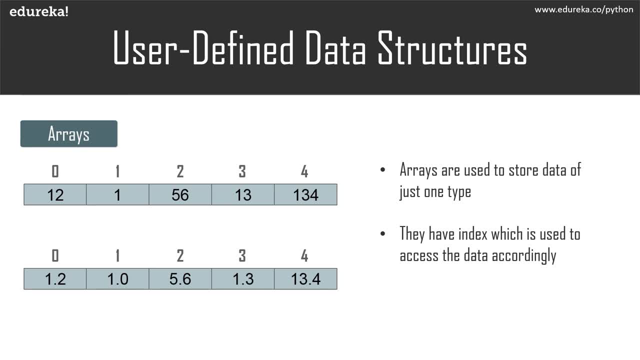 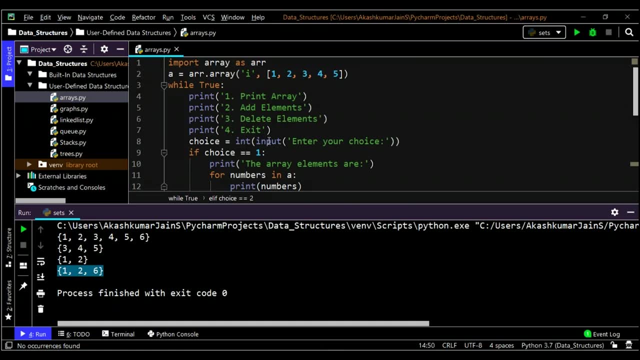 So I hope you're clear with this. Let's move ahead to the program that I have prepared for all of you guys, and we will not be typing these because it takes a lot of time, So let me just show you the program for now. 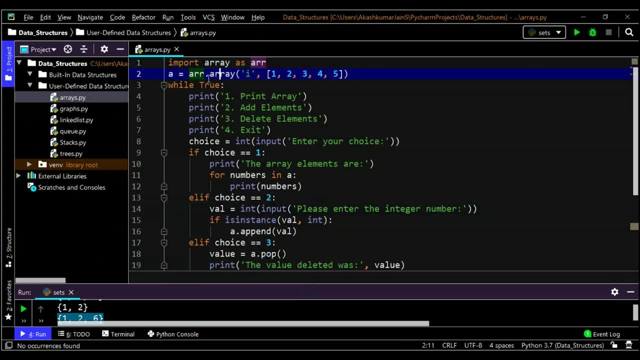 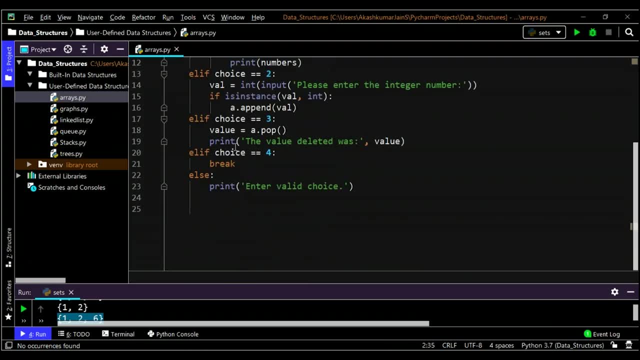 So I have imported the array as a RR and I have created an integer array and passed 1, 2, 3, 4, 5 as the elements, And then I have the while loop in which I'll be performing the certain operations. So let me go ahead and run this program for you. 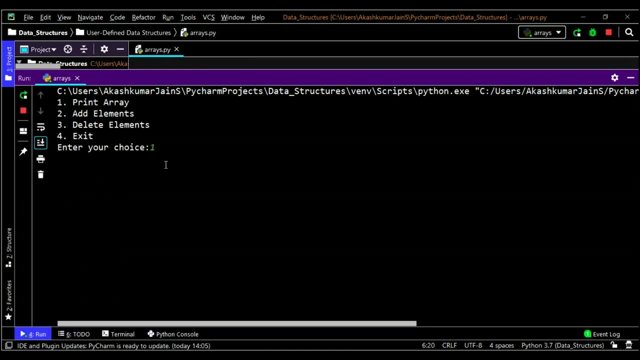 Yes. So, as you can see, let me write my first choice, that is, printing the array. So I already have an array which is 1, 2, 5. right now Let me go ahead and add an element. Let me see: this number is 10.. 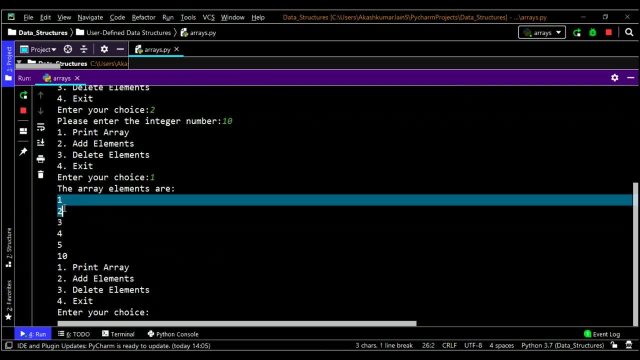 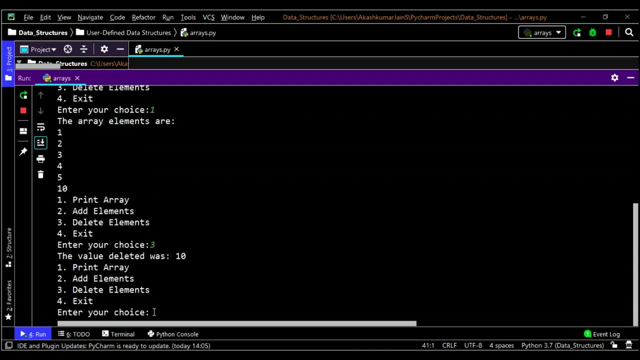 Let me print the array again. So it is 1, 2, 3, 4.. 4, 5 and 10.. Let me see: delete the elements. So the value which was deleted was 10, and let me just exit out of here. 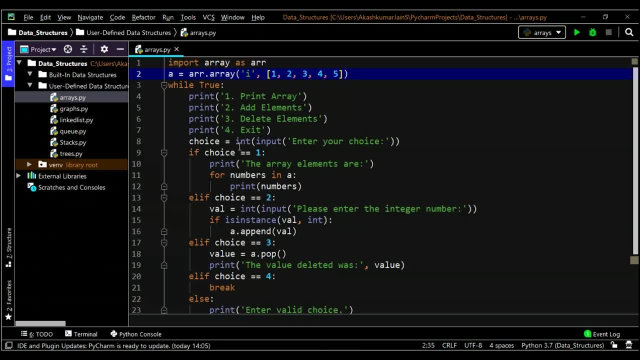 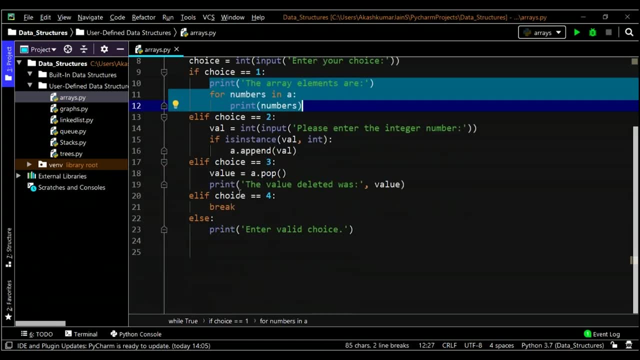 That is basically what an array is. So, as you can see, let me just explain the program. So I take the choice and if the choice is one, I am going to print the array elements. if the choice is to, I will be adding the integer elements. 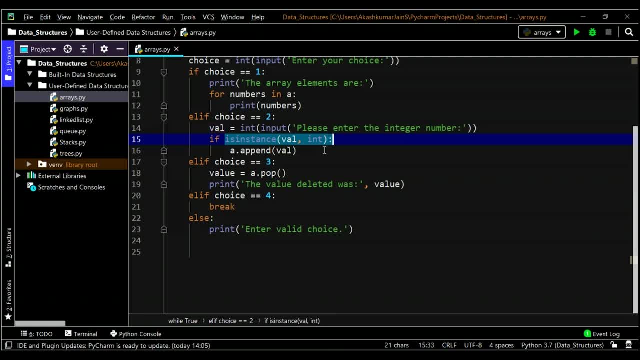 and I will make sure that the integer element is only taken over here, else the program ends over here. Then I have three, which is to pop the element, and I have four, which is to break out of the while loop. If I enter any other choice, it will say that please enter a valid choice. 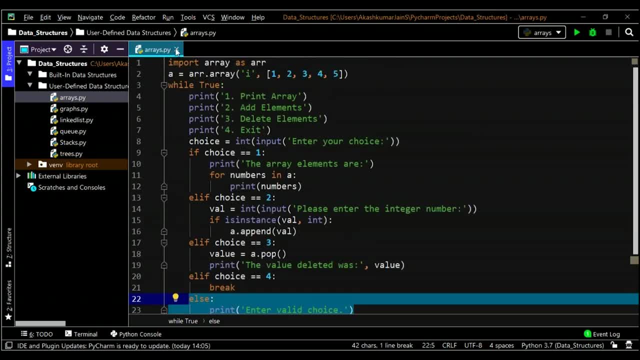 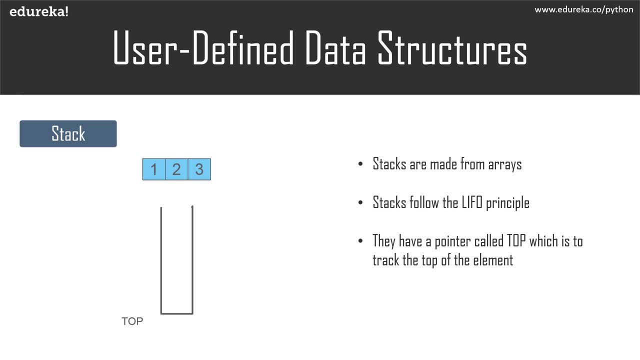 and keep running in the loop itself. So that basically wraps up arrays. Now, once we have understood what arrays are, let's move ahead with stacks. As you can see, stacks are made from arrays and they follow the LIFO principle, which is the last in and the first out. and how is? 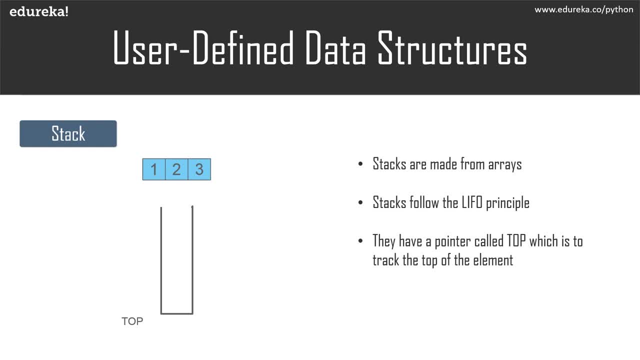 that being taken care of. it is being taken care of something called as the top, which is the pointer to track the top of the element. So let me show you how this works. We have some elements, which are 1, 2, 3. now to add elements. 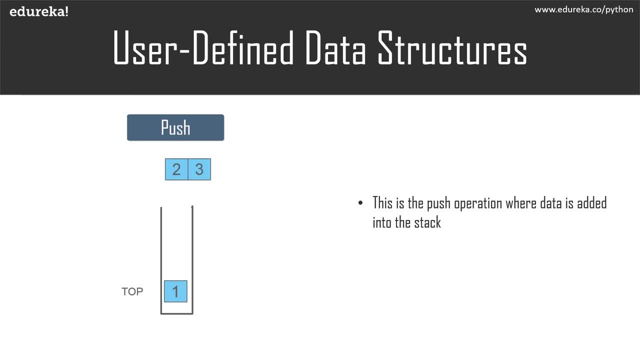 into the stack, It is called as pushing, and to delete elements, It's called as popping. So let me show you how a stack basically works. So I push one. So, as you can see, one is being pushed to, will be pushed, and top is basically pointing to the top. 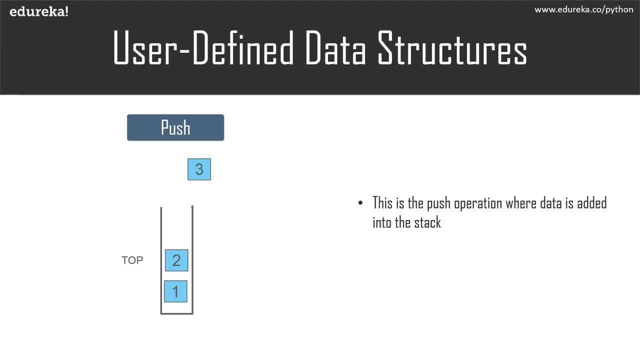 Top of the elements. So whichever element is at the top, top will be pointing to it and three will be pushed. Now, what happens on? if I want to delete it, I just say pop, and three will be popped out and top will be pointing to value number two. 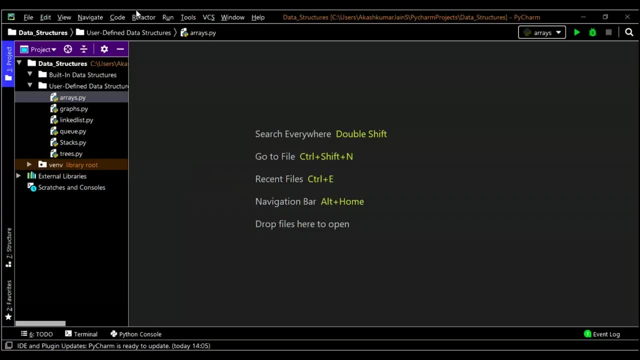 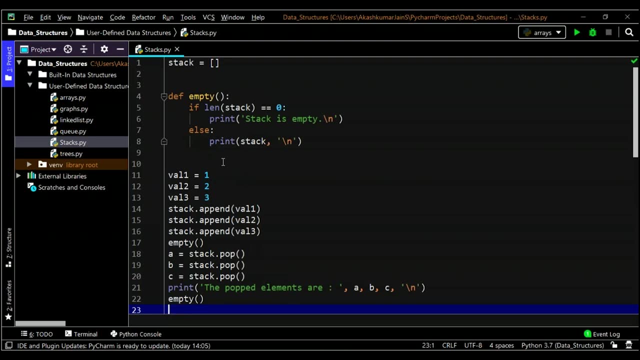 So this is basically what a stack is. Let me go ahead back to the program that I have prepared for you guys. So for the stack program, I have prepared it in two methods. It is either Using the normal lists or I have defined it using a class. 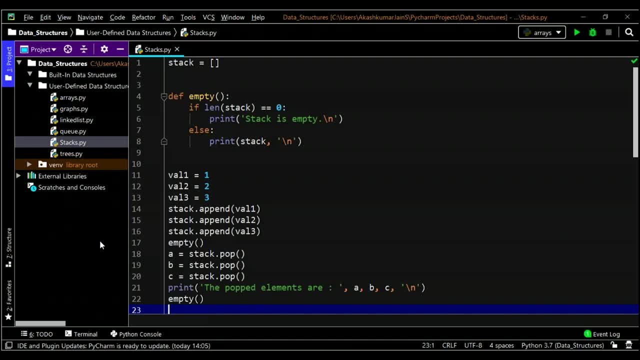 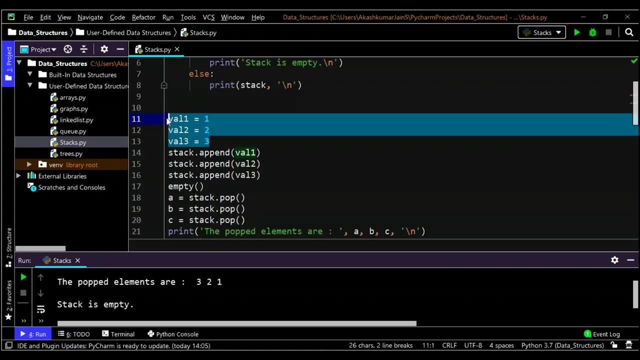 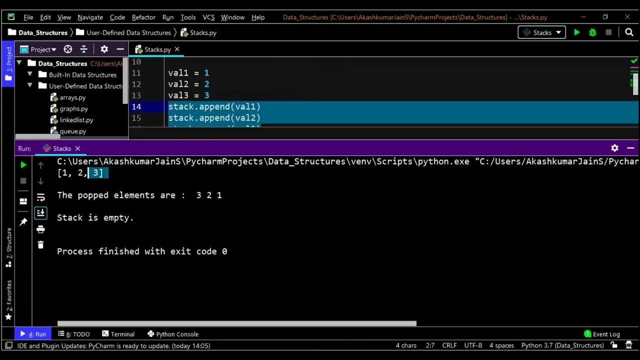 So let me just run it according so that I can show both of it to you. Yes, as you can see, I have three values over here and I am appending all of these to the list. So now my stack is having the values 1, 2 and 3.. 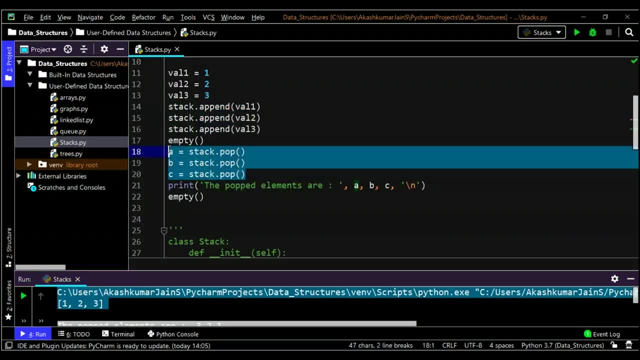 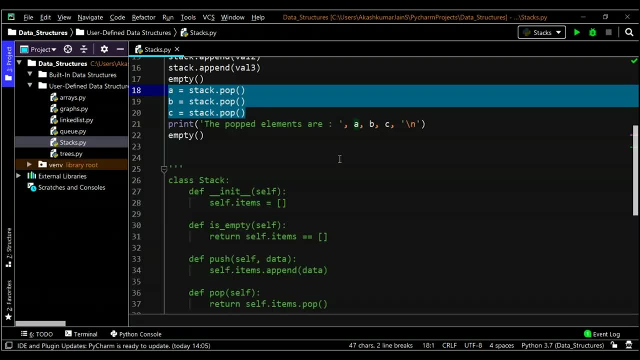 Let me go ahead and pop these elements. That's what I am doing over here. So 3, 2 and 1 are being popped, So the stack is empty. This is not that interactive. So to make it much more interactive, What I had done is I have used classes. 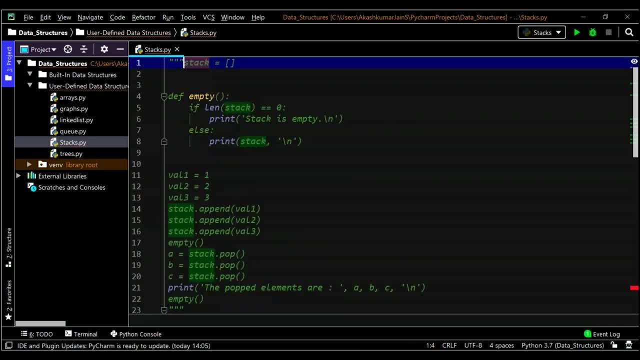 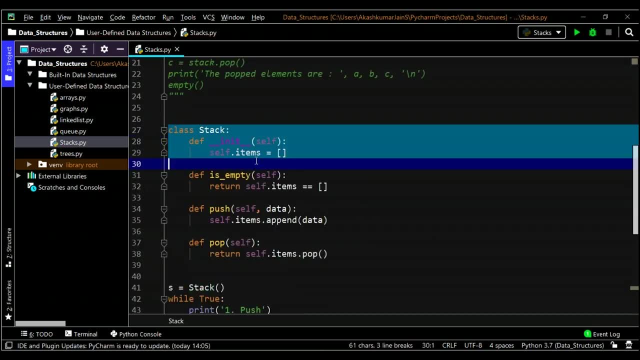 So let me just show that program to you right here. Yes, So this is the class of the stack. I have items, then I have returned self dot items if it is empty, and I have the push and I have the pop functions. So I have created a object over here. 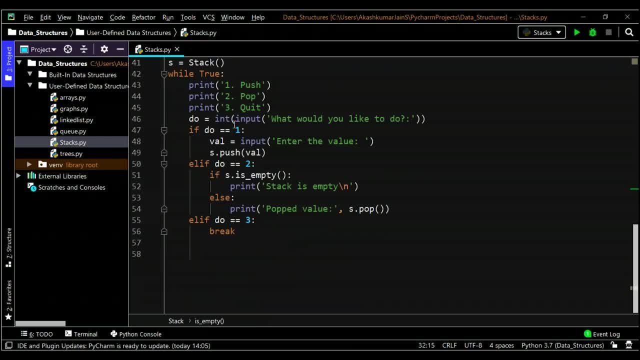 and I am asking the user. So let me just go ahead and run. This is the same as what I had done for the other program. I have asked the user for this choice. So I either push or I either pop, and I either pop out the thing. 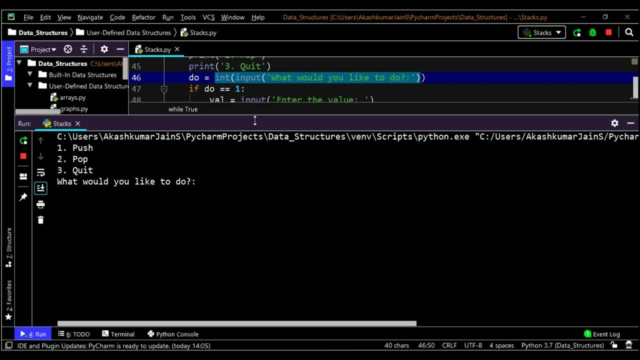 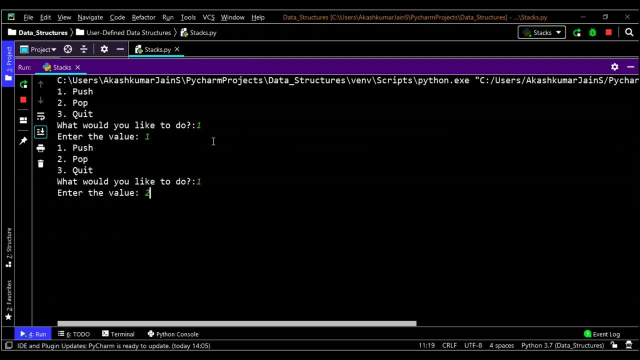 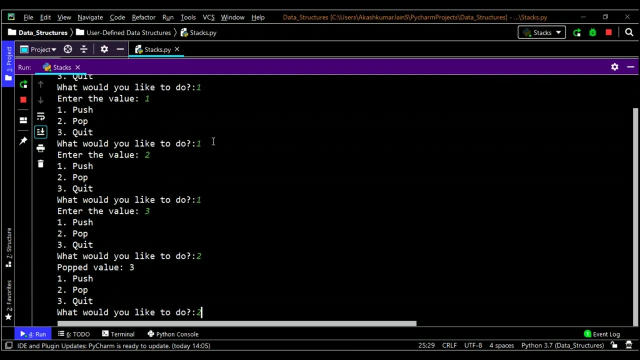 Let me run this program. Yes, What do you want to do? Let me push a value. one is being pushed. Let me push on the value 1, 3.. So let me pop the value. So the pop value is 3 over here. 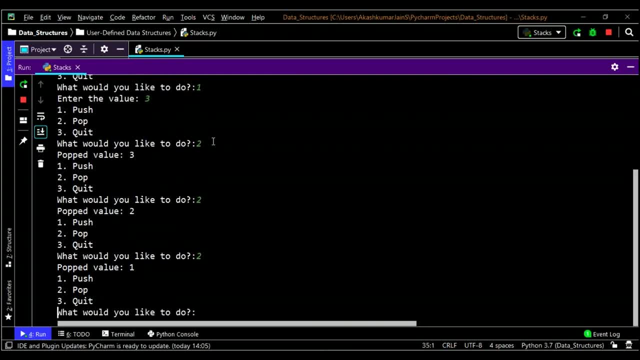 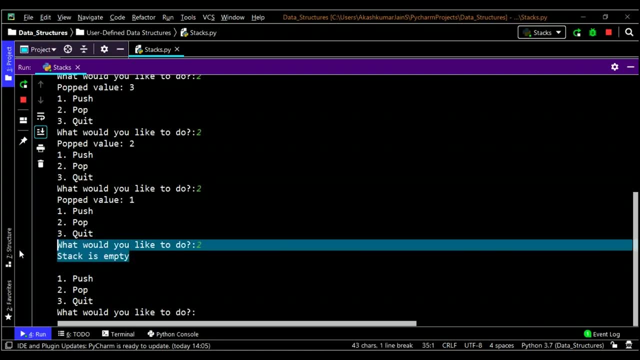 Let me pop another value. The pop value is 2.. Let me pop the value. pop value is 1.. Let me pop it again, even though there is no item. Let's see what happens. It shows me that the stack is empty. 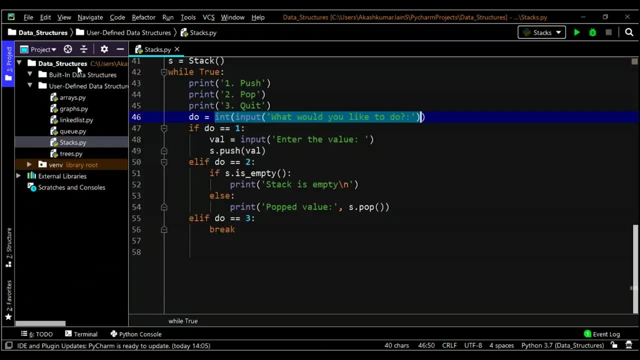 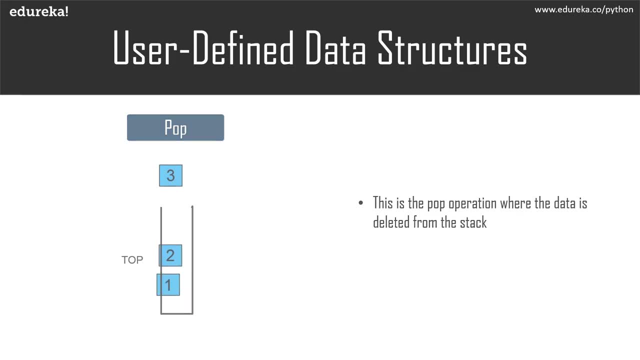 Now let me quit from you. That is basically how a stack is being implemented in Python. Let me close this for you. Let's move to the next data structure. So the next data structures are queues. So queues are basically the same as stacks, with one difference that they follow the FIFO principle. 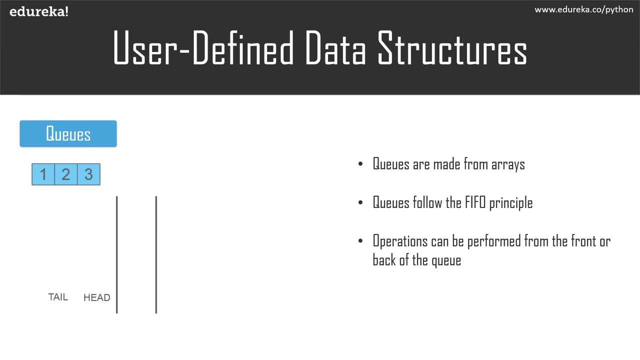 meaning that whatever element comes first will be the one that will go out first, and operations can be performed from the front or the back, which is basically the tail and the head. So let me show you the enqueue process, which is to add elements into the queue. 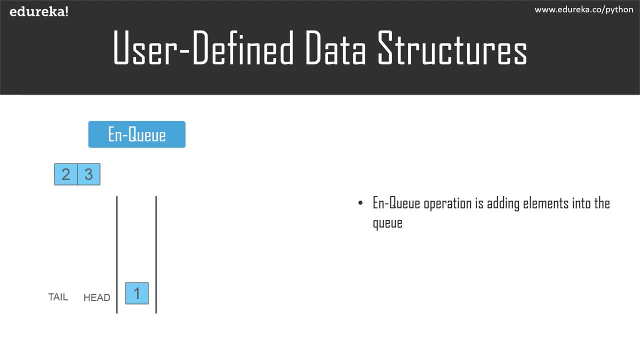 So one is added. as you can see, we have two pointers over here, which are head and tail, and head and tail are now currently pointing at one. Now let me add to, so tail is at two. Let me add three, So tail moves and points over to three. if I want to dequeue, dequeue. 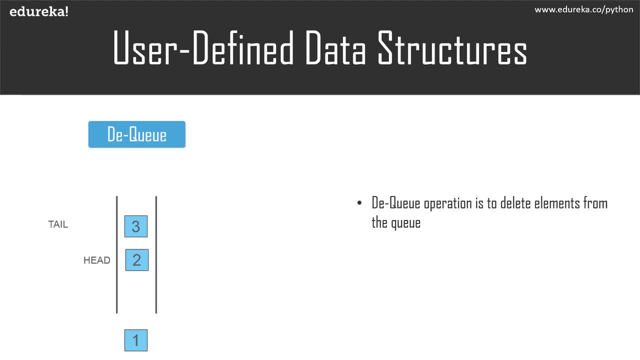 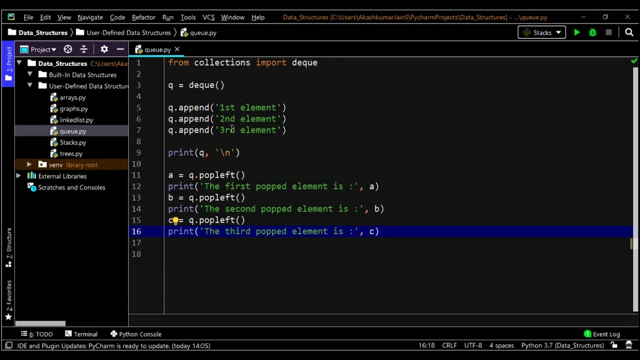 is basically to remove a particular element. So one comes out and the head is now pointing at the element number two. So let me show you the program that I have for you guys. Yes, from the collection I am just importing dequeue and I am appending the elements. 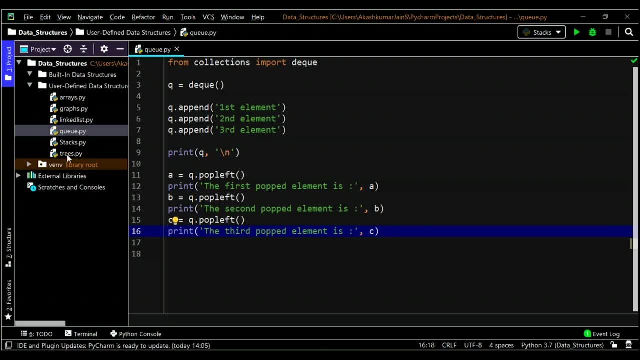 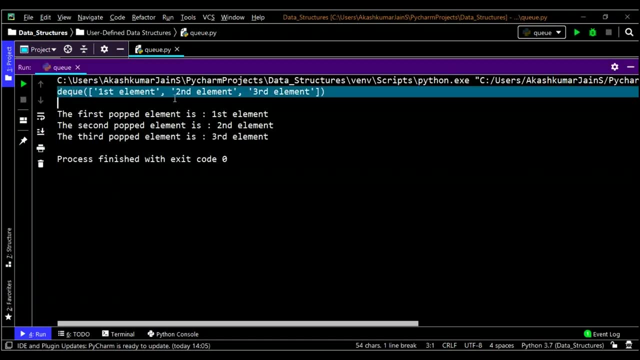 accordingly and then pop left, pop left. So let me run the program So you'll understand it better. So, as you can see, I have first element, second element and third element over here. So the first pop element is one, the second pop element is two. 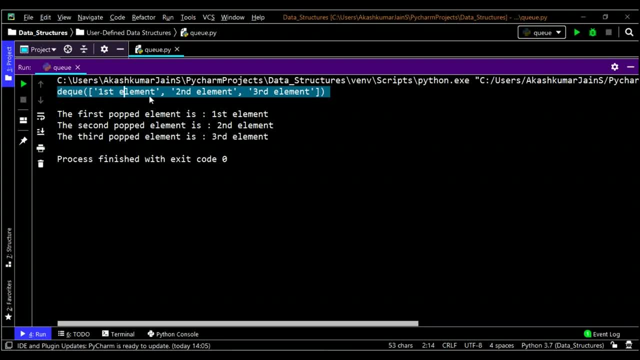 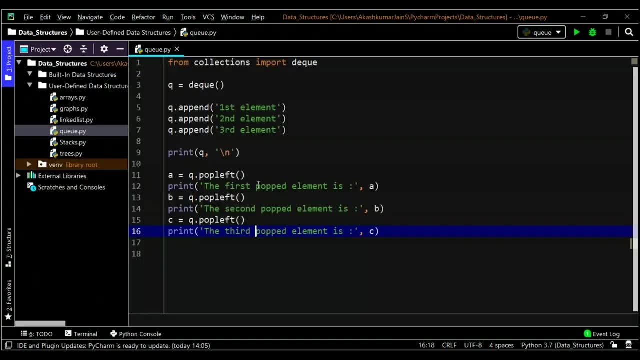 and the third pop element is three. So first element was first to come in, second and third accordingly, and then first element was what was popped out. So that, basically, is a queue for you guys. So now that we have understood what queues are, why don't we? 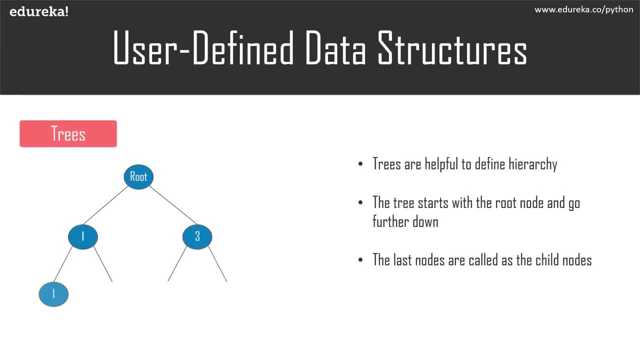 move ahead with the next data structure, which are trees. trees are basically used to define the hierarchy. Now, where would you use a tree? trees are basically used in your HTML pages, which are used to define what tag comes under which other tag, and so the first HTML tag is called: 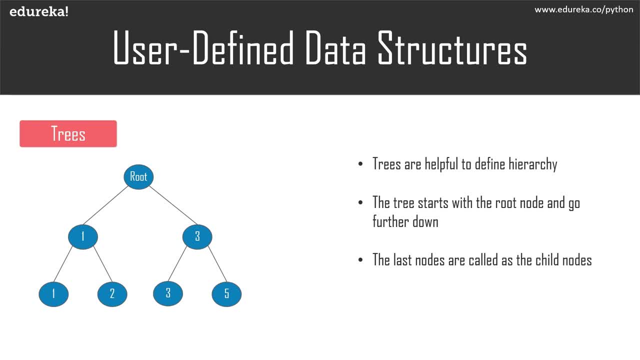 as the root, and all the other tags which are inside the HTML tag are called as the leaves or the children of the parent node. So let me go ahead and show you the program. Yes, So as you can see, I have the class node over here. 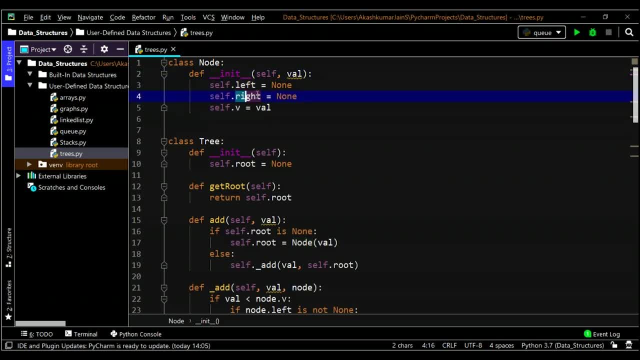 which is basically saying that we have a left and the right. What does the left and right mean? It's basically that, to the parent, you have a left child and the right child. So basically, here I am showing you the demo for binary tree. 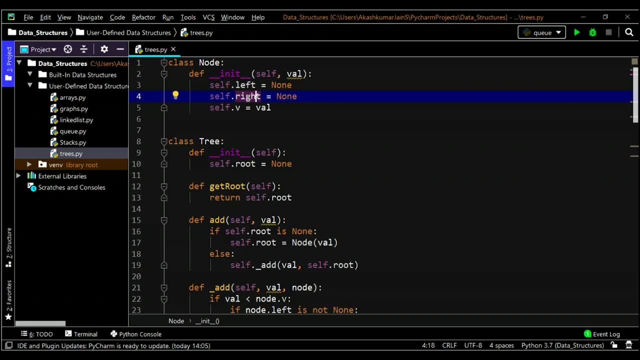 So the left child will be element which is lesser than the value of the root node and right child will be value greater than the root node and self-taught we will be the value. So I just say that initialize the root with none, And if I want to get the root, 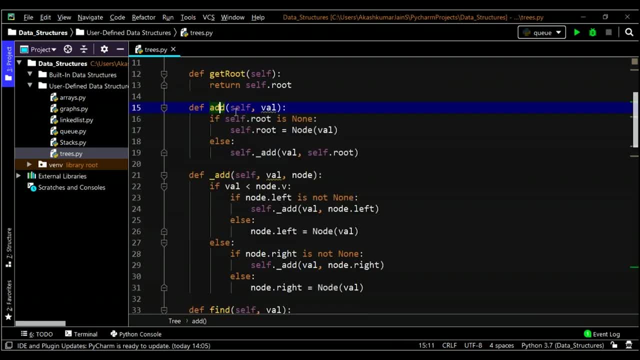 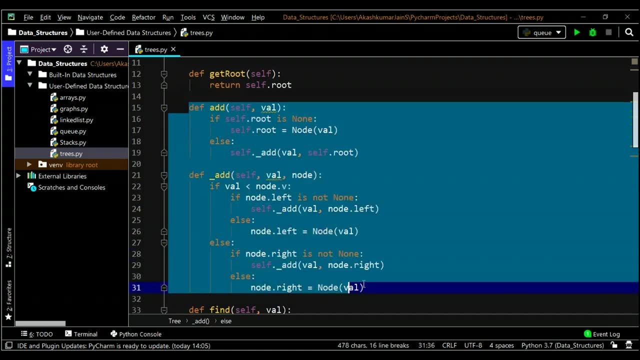 I just say that self-taught root and return the value for it. So if I want to add a particular node into the tree, I have two functions over here which are basically define, add and define underscore add. what happens over here is if the tree is empty. 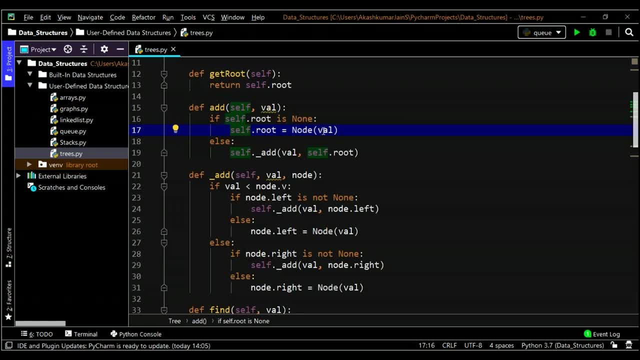 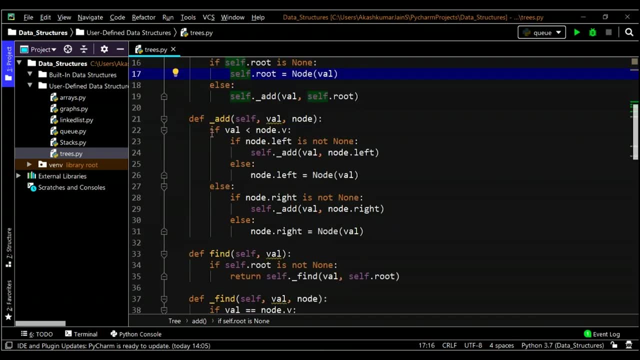 I will basically take that particular node and convert that into the root. If it is not, then I will recursively keep calling the function which is happening over here. So if the value Of the root is less, I perform this function, and if it is greater, I perform this function. the same goes. 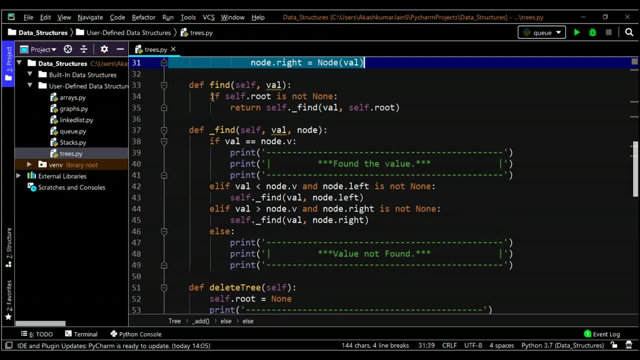 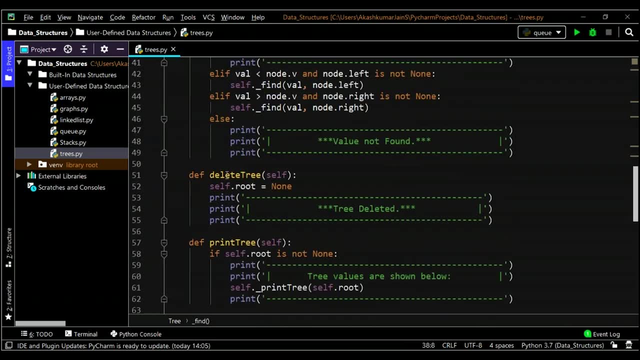 for find. also, I will just say that if it is not none, I will recursively find the value, or else I just say that it is not found accordingly, So delete the tree. So I will just say that the self-taught root is equal to none. 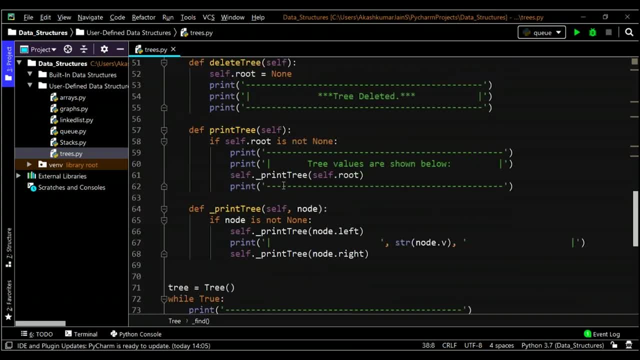 and basically delete the tree, And then, if I want to print the tree, I use this function over here, which is, if it is not none, I just show that these are the tree values and accordingly find out what are the values of the trees. 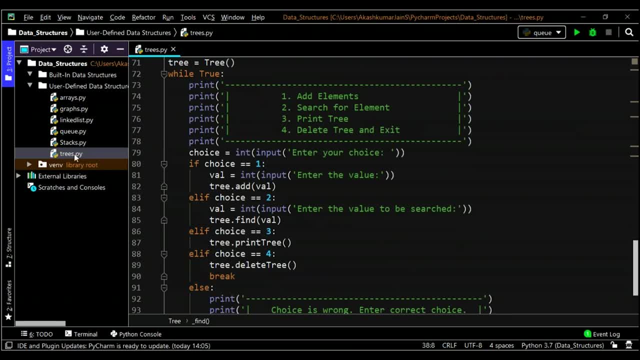 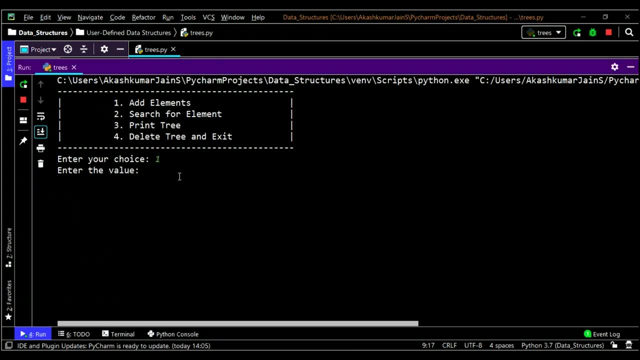 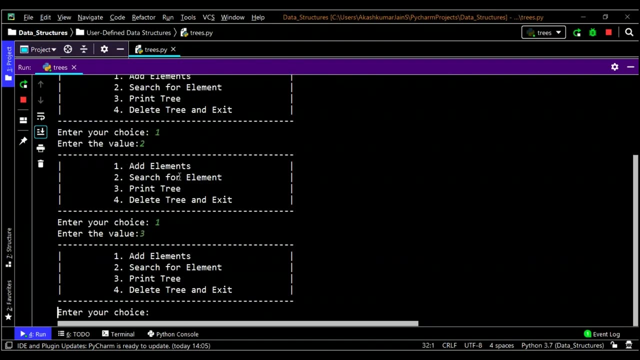 and I have made this interactive, meaning that the user has to add inputs. So let me run this program So, as you can see, I will add elements. So I will say: add one, add elements, add to add an element, add three, add an element, add for add an element. 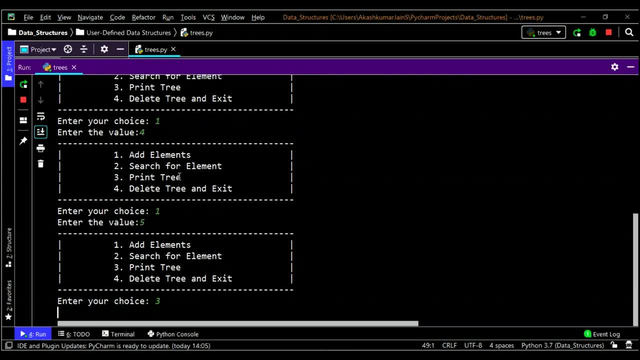 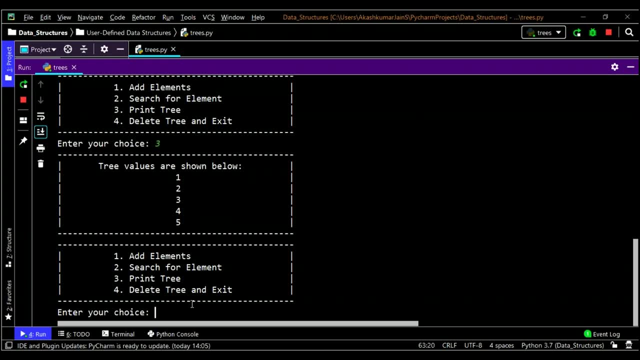 and add five. So let me print the tree for you. So, as you can see over here, the tree values are 1, 2, 3, 4 and 5. let me now go ahead and search for an element. So let me say I am searching for three. 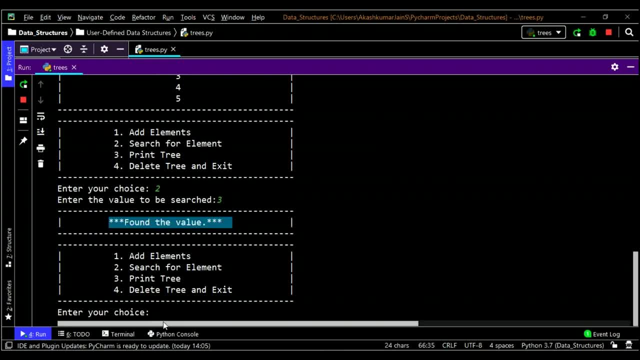 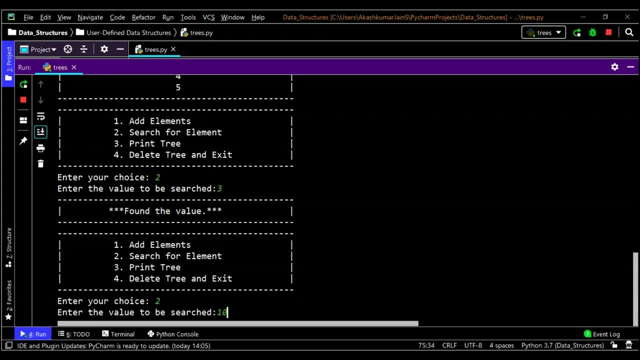 So it shows that it has found the value into the tree. Now let me search for something which is not inside the tree, Right? So let me say that I want to search for 10 or 19 or anything. It sees that the value is not far. 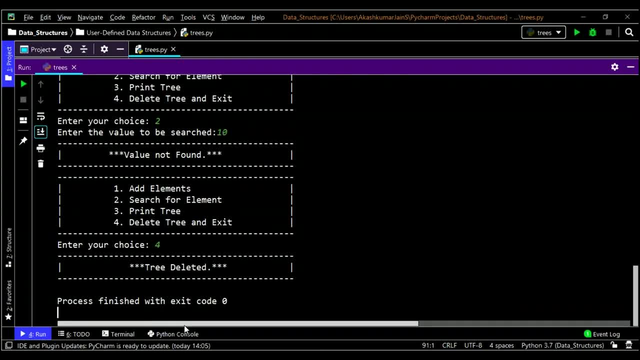 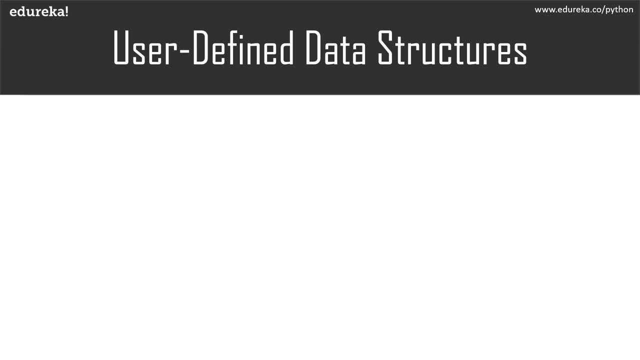 Let me go ahead and delete the tree and exit. So the tree is deleted and the program exits. So that, basically, is what a tree is for us. Let me move ahead with the presentation and the next data structure, which are linked lists. So the linked lists are made up of two fields. 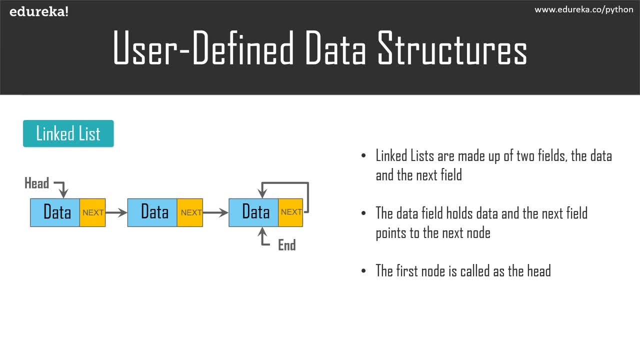 which are basically the head, and the pointer, which is pointing to the next node. We have head, which is the first node of the linked list, and end, which is the ending of the linked list. So the first node is called head and accordingly it has two fields, as I told you. 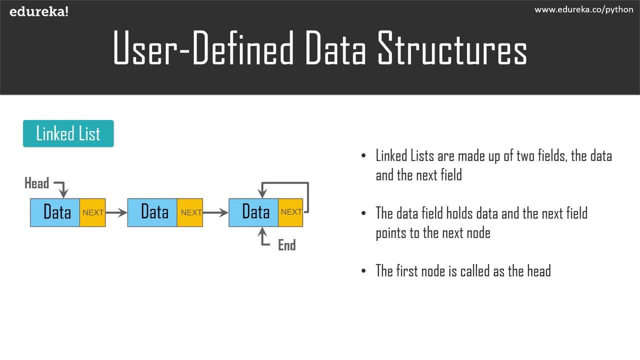 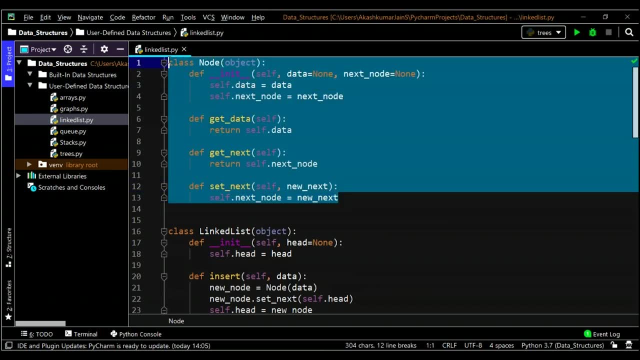 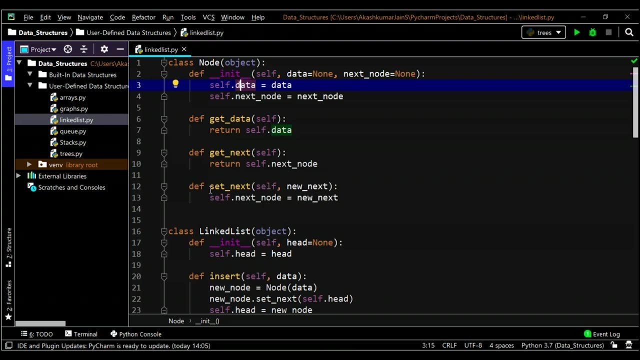 that it is used for holding the data and the pointer to the next node of the linked list. Let me show you the program. So I have a class called as the node, which is basically self dot data and the self dot next node, and to get the next data and set the next data accordingly. 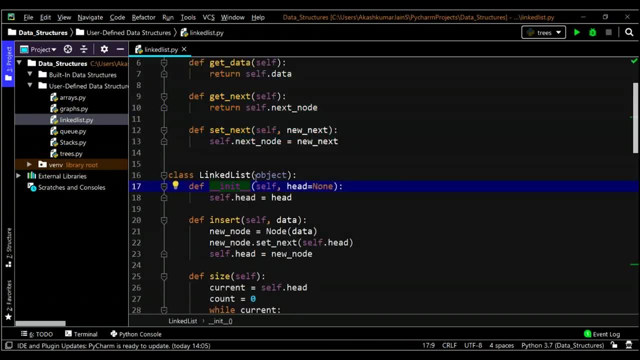 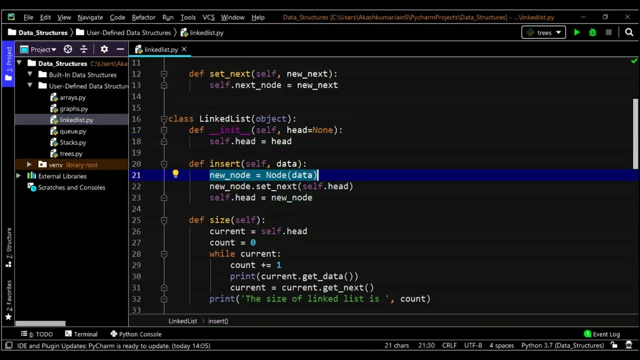 I use these functions right. So I am creating a linked list object. So I just say that the self dot Head is equal to head. then I have new node is equal to basically to insert the data accordingly. Then I have the size over here. 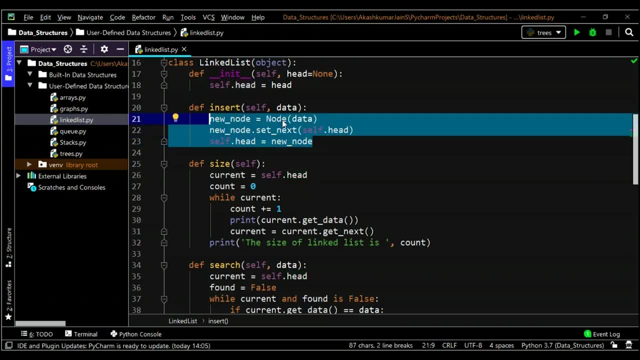 So here what happens in the insert is basically: I have the new node is equal to node of data, I am creating an object for it and then I am setting itself accordingly, and then self dot head is equal to new node. So this is what happens in the insert function. 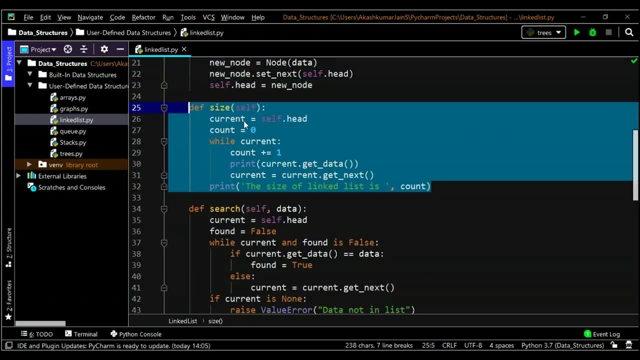 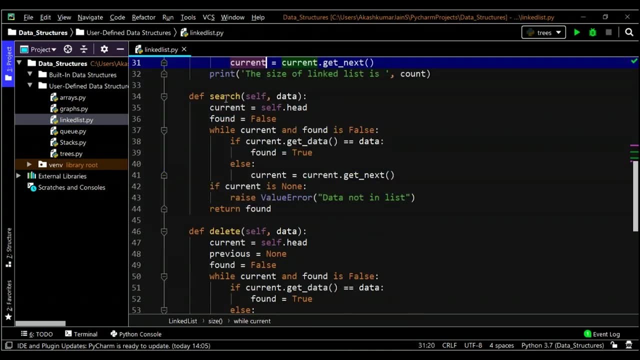 Then I have a function which is used to find out the size of the linked list, So it basically Traverses through all the data elements in the linked list and gives me the count of it. Then I also have a function which is used to search the value. 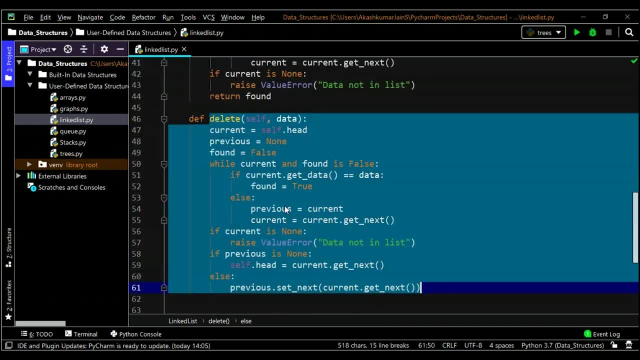 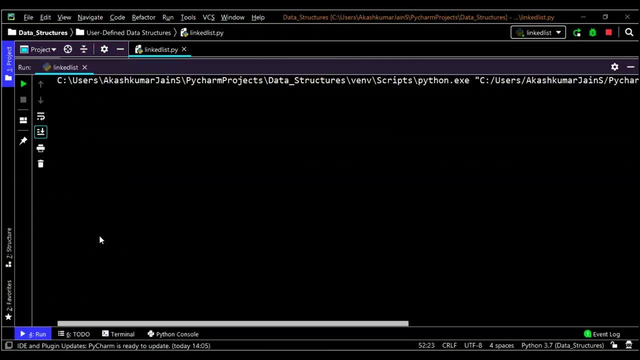 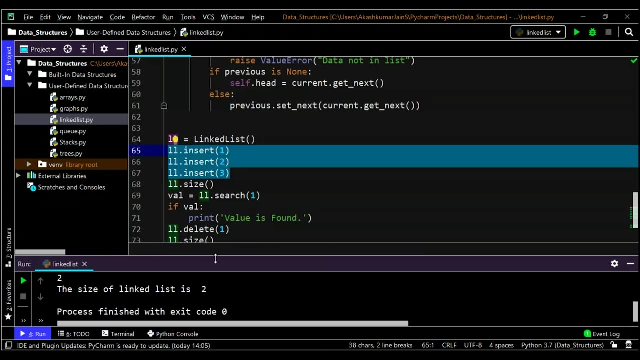 and then I have element which is used to delete the particular data in the value. Let me just go ahead and run this for you. Yes, So as you can see, I have three elements in my linked list, that is, one, two and three. That's the reason I have got one, two and three over here. 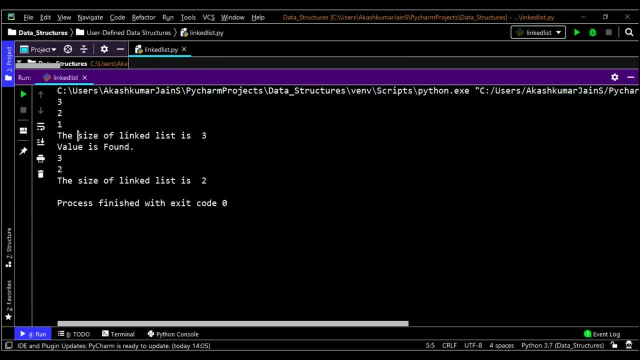 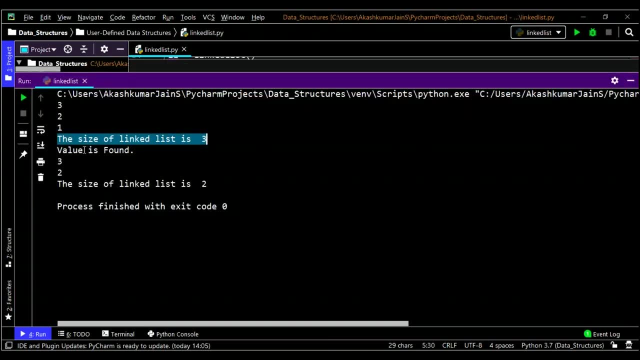 And then I am finding the size of the linked list. So to find the size of the linked list I just had, the size of linked list is three right now, and then I am searching for one in the linked list and I do get the value in the linked list. 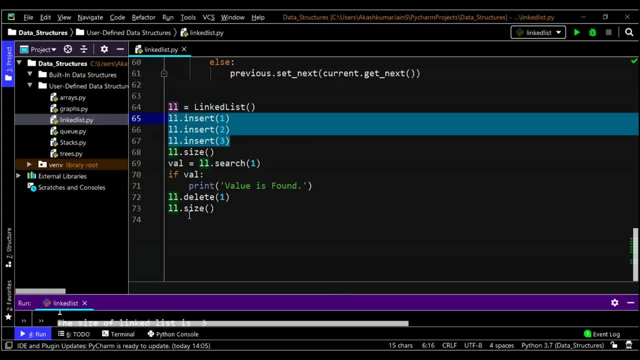 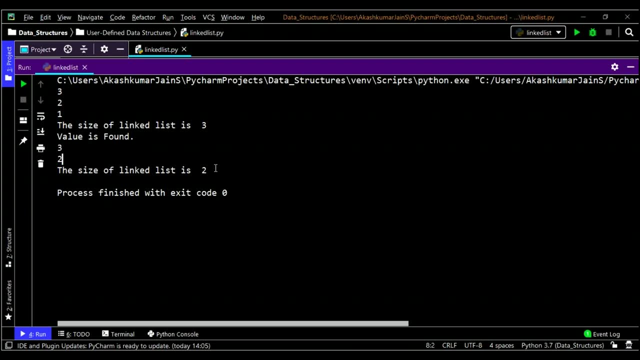 So I have value is found and then I have delete one and the size. So I just want to say that I want to delete the first element. So I deleted the first element and when I print I get three and two and the size of the linked list is two right now. 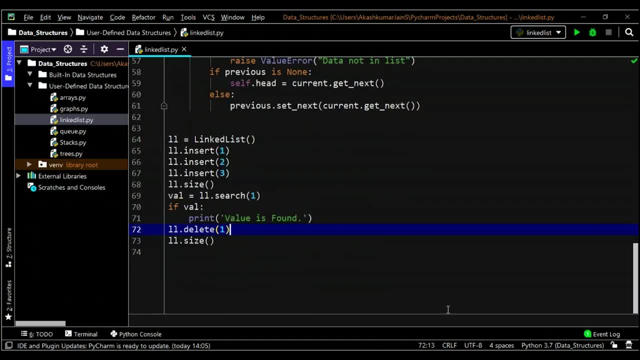 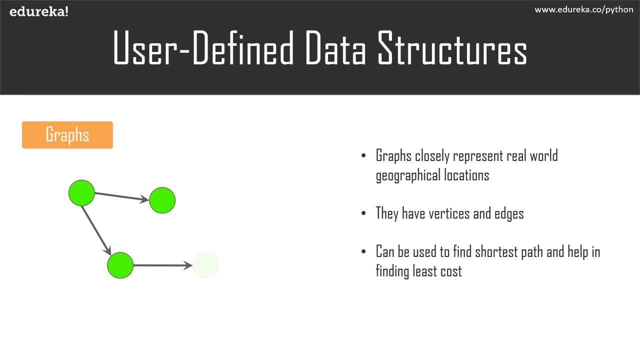 So that is basically what a linked list is in our particular example. Let me go ahead with the next one, The last. a data structure that we have is graph right now. So graphs are basically used to show vertices and edges. So vertices is basically showing you a particular location. 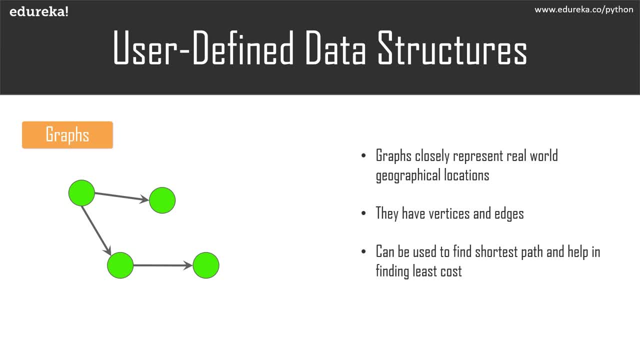 So where we use graphs is basically to represent geographical locations, right, So we have the green over here, which are called as the vertices, and the edges are basically the arrows from where we move from one part to the other, So these can be used to perform certain calculations. 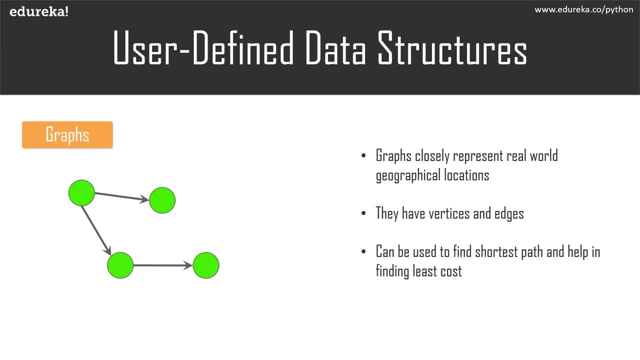 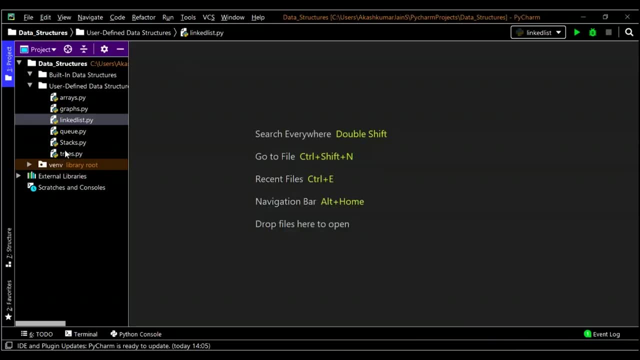 where we can find the shortest path and all the other features, wherever you can find it on a particular map. So let me show you the program for this. Let me close this. Yes, so I am just having the default dictionary which is being imported from the collections. 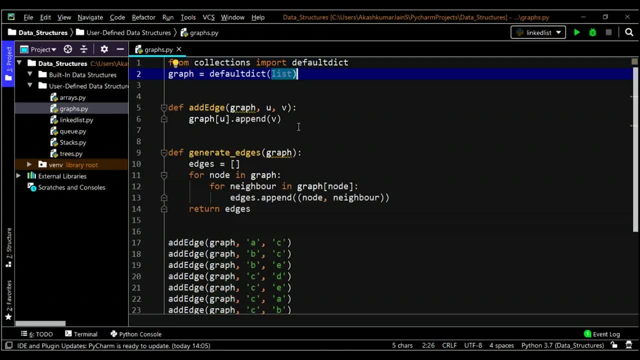 and then I have: graph is equal to the default dictionary of a particular list. Let me just say that I am adding an edge. So to add the edge I have to have a particular element and the word is: and so this is what is the function. 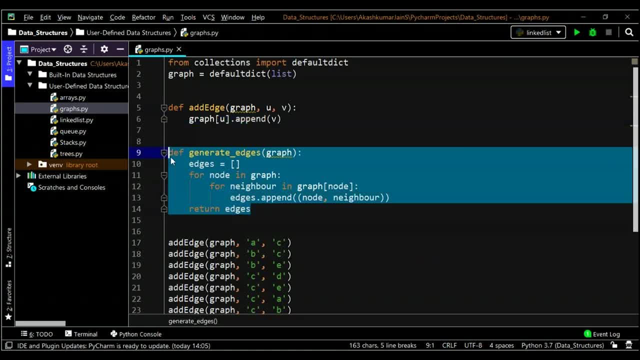 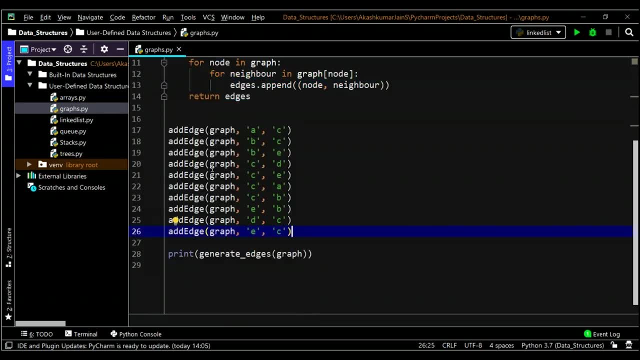 that is used to do that, and then I am to generate the edges. So basically, I'm just showing that to a particular element There is an edge that exists. So I have A to C, B to C and so on. This is basically my graph that I have drawn. 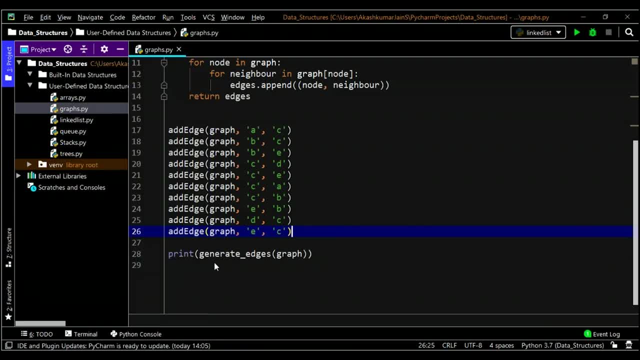 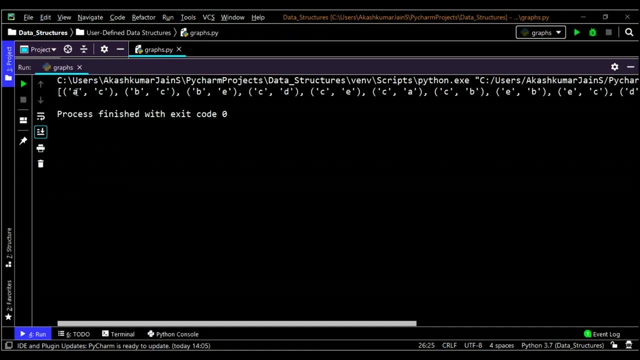 So let me show the output to you guys. So what output that I'm going to get over here is basically to show all the different edges that are between one to the other vertices. So a is connected to C, B is connected to C, B is connected.